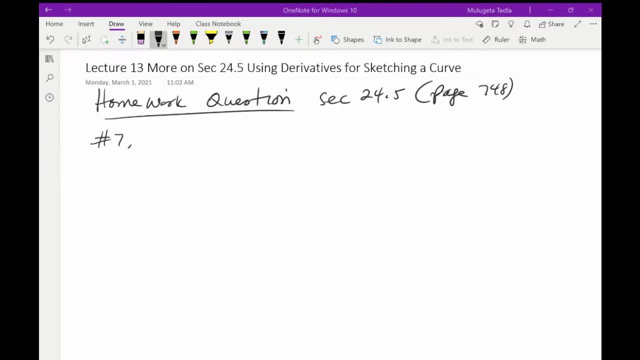 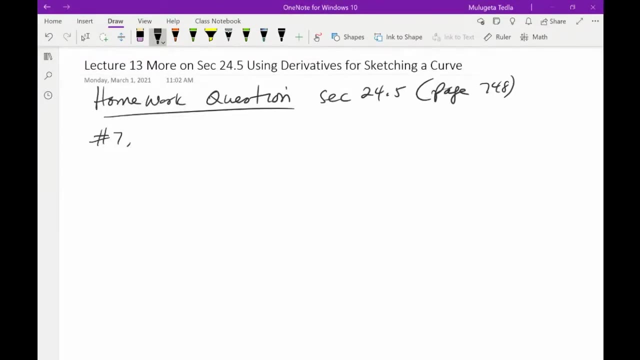 eleven, i will choose one and i'll do number fifteen. two questions i will do okay, because the whole class will be over if we just request this. you understand? so i think from seven and eleven they are of the same category so i will do probably eleven. the same, the same function. anyway, number seven and eleven are the same. they use the same function. so 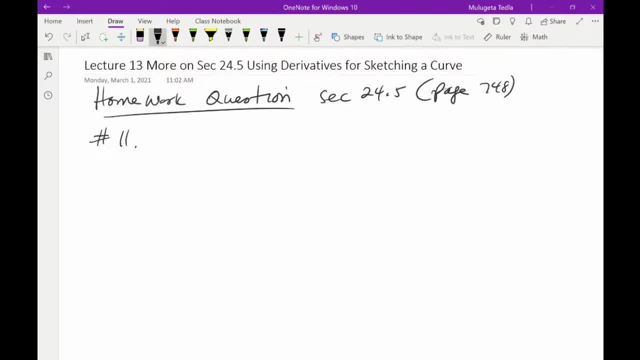 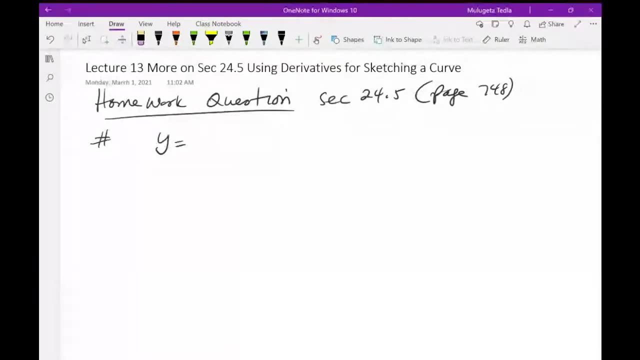 i would rather have seven, eleven, because they ask more questions than that number eleven, but the function is the same. why? equal to uh oh, fifteen is the same, so i think let me do fifteen. okay, what is that? uh uh, strawberry number fifteen is number seven number. uh uh, number seven number. 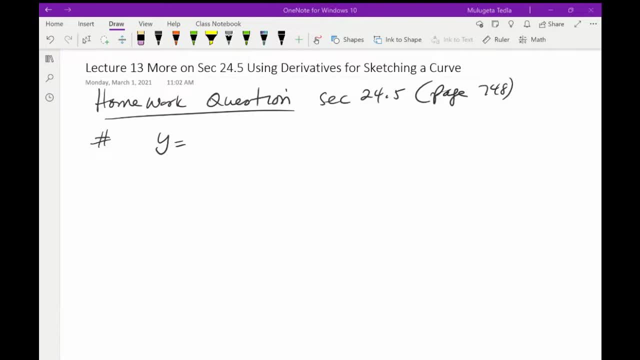 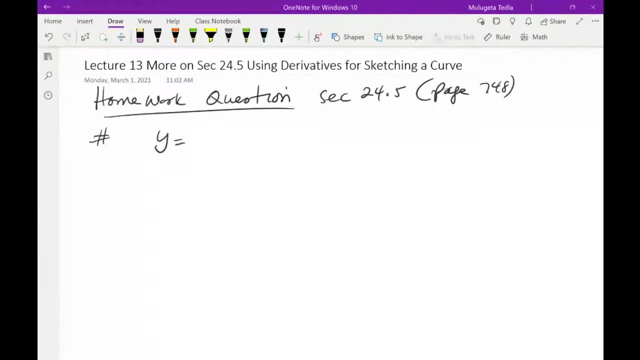 eleven, number fifteen, are the same question, except that, uh, number fifteen is more, uh, more, it has more, more questions to it. so you can sketch the graph. so i will pick number fifteen, which will cover seven and eleven. okay, number fifteen it's saying: use y equal to 2x cubed plus 3x squared, minus 36 x minus. 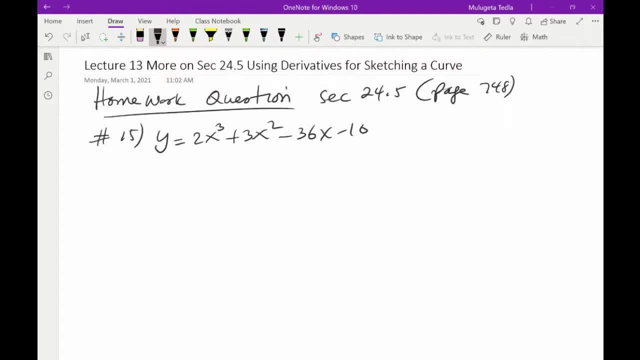 10.. okay, so find uh first number seven states: find the increasing and decreasing. number seven, uh, find the intervals of increasing and decreasing which we we're going to need anyway for sketching graph. number eight, okay, no, number 11, rather, number 11 says: find the local point, find the local max. 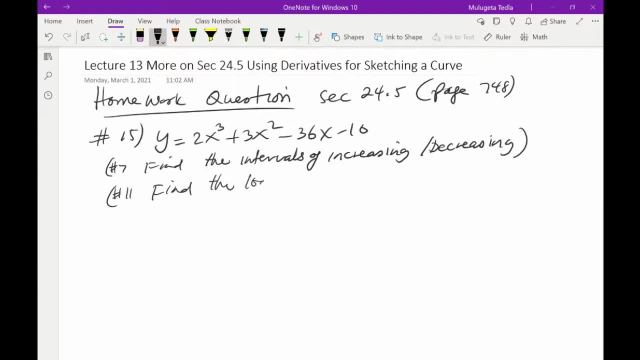 and local minimum, local maximum and minimum points. all right. number 15: find the values of x, which the function is, concave up and concave down, and any points of inflection. this is something we're going to do, okay, so now i get it, so i think i will do. number 11 period. 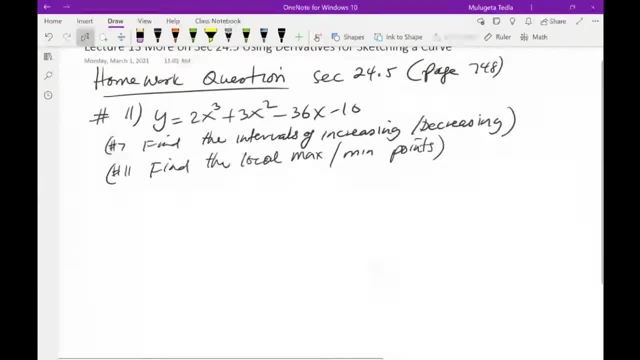 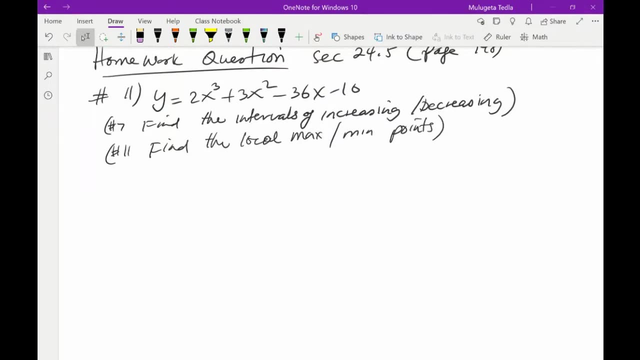 i will. i won't do number 15 because we haven't covered it yet, so we're gonna do. i'll give you definition and all that before i i do example. okay, so i will do your number 15, strawberry, but you just have to wait for a little bit, okay? so, uh, as part of number seven: 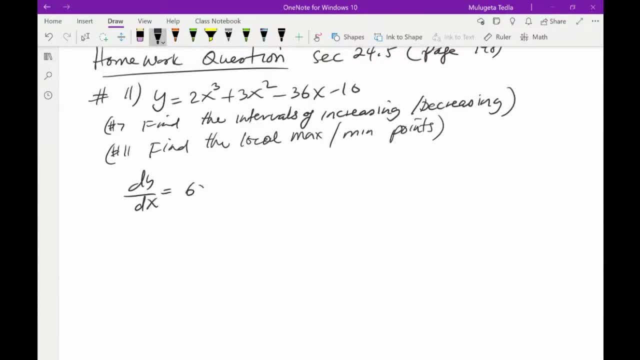 we find dy by dx, which is equal to 6 x squared plus 6x minus 36, and we said that the zero, it gives me critical numbers. okay, then, how do you find the critical numbers? you, you, you find the derivative, you create the zero, and then, of course, you can factor six x squared plus x minus, uh, six equal to zero. so that's. 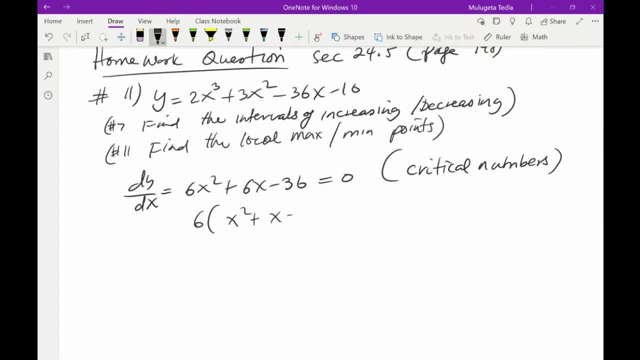 fine, zero. so then, before i do one- that's critical numbers, um, then i do one, so you find the critical And then you can factor x squared. This part can be factored as x times x, and then 3 and minus 2, because 3x minus 2x is x, which is the middle term. 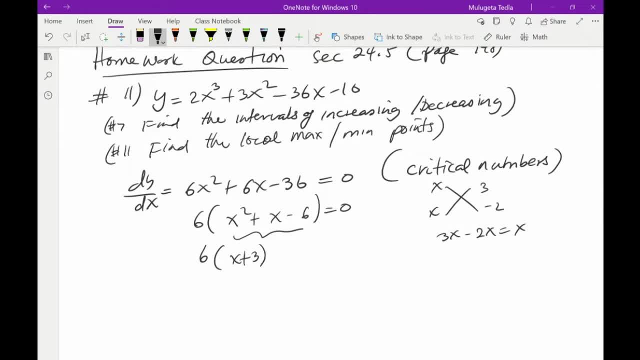 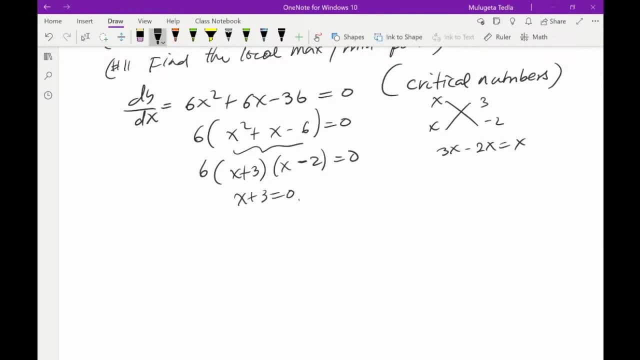 So it works 6 into x plus 3 and then x minus 2 equal to 0. So therefore, x plus 3 equal to 0, x minus 2 equal to 0, is x equal to negative 3 and x equal to 2 are the critical numbers. 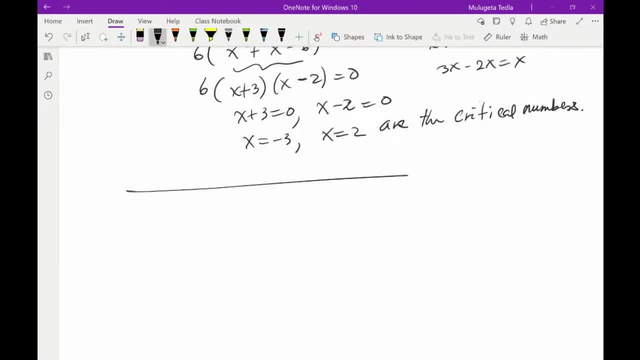 Okay. so therefore, now we're going to split. The critical numbers are x coordinates of the maximum and minimum points. You know what I mean. These are almost almost there for the maximum and minimum points, But that's number 11.. But let's find the intervals of increasing and decreasing. So we do sine chart, Sine chart. How Well copies. 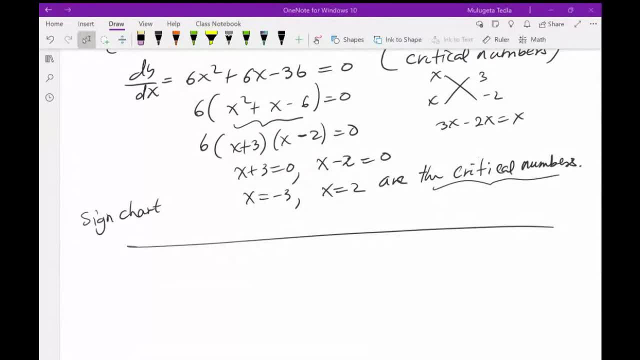 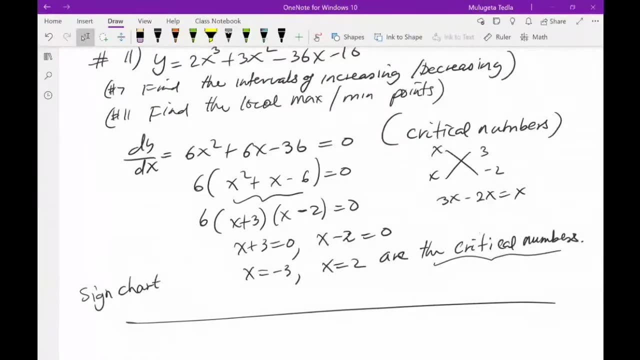 Is there any question? Yeah, So with that, In this case, the negative 3 and the negative 2 is interchangeable, right, Like it could be negative 3 and then 2, or it would be negative 2 and plus 3.. 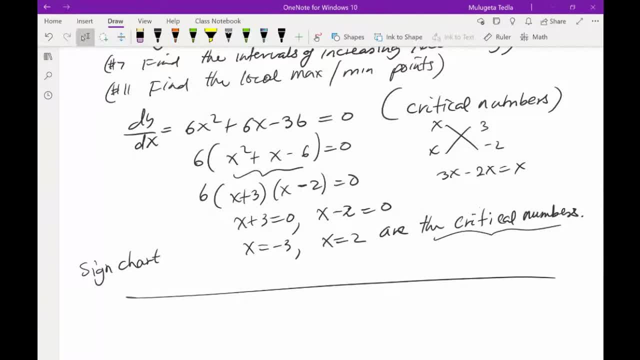 No, No, it can't be. It is actually the way they are. You cannot have negative 2, as If you plug negative 2 in here, it won't be 0. They're not interchangeable. The sine is not. 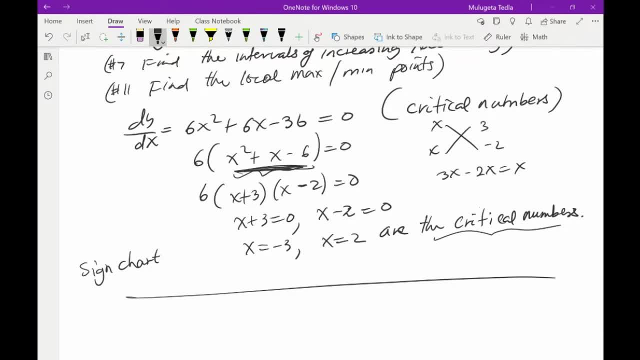 Okay, thank you. Yeah, you understand what I mean, that what we're looking is for something for the derivative to be 0. If I plug negative 2 in this, I will never get 0. So it's not really a solution. 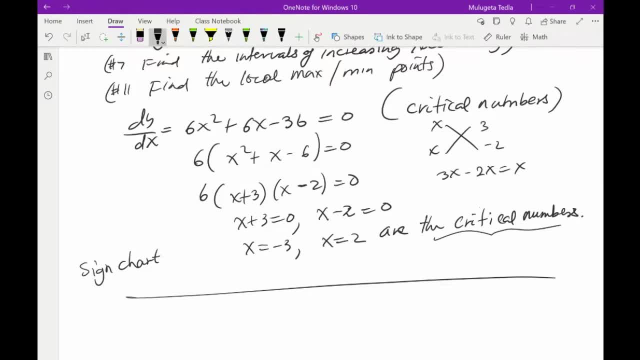 So, therefore, the only thing is x plus 3, x minus 2 and number 6 multiplied 3 of them is equal to 0.. We know that 6 cannot be 0, but either x plus 3 equals 0 or x minus 2 is equal to 0. 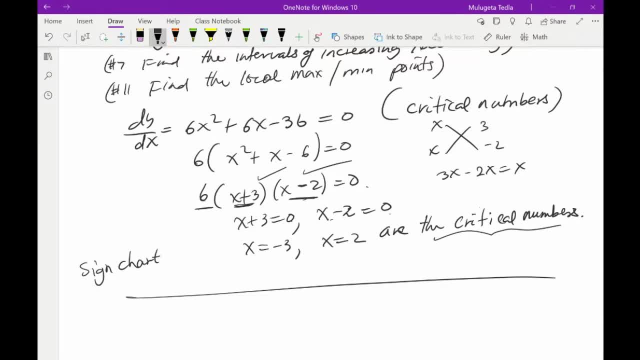 When I do that, what I get is x equal to negative 3 and x equal to positive 2.. We cannot use x equals positive, 3, x equal to negative 2.. And you can easily check that this is that. those are not the solution. 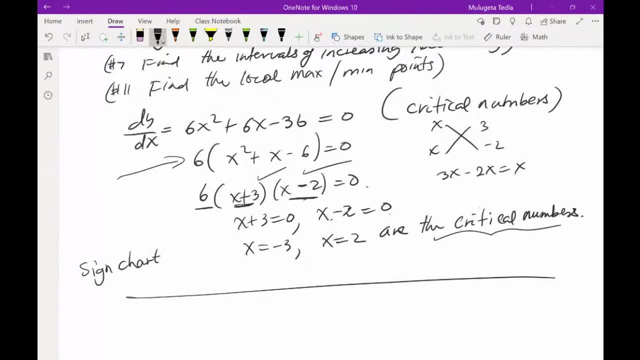 Because when you plug them into the derivative- which is right here- they will not give you 0,, so they can't be a solution. For them to be a solution, They should satisfy the equation you're solving, And they don't satisfy. 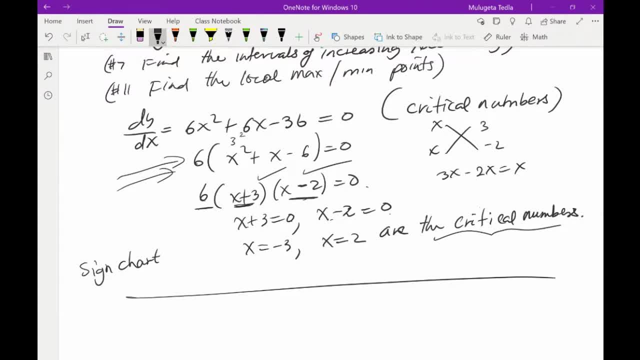 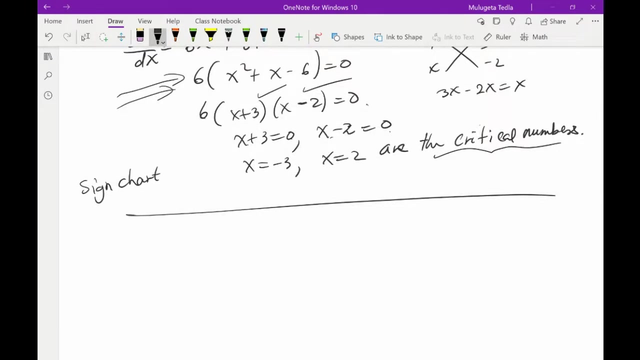 If you plug 3 here, positive 3 squared plus positive 3 is like 12 minus 6 is not 0, can be 0, so they cannot be anything else except negative 3 and positive 2. the chart, okay, is split to a few, a few intervals. there is negative 3 as a boundary line, there is 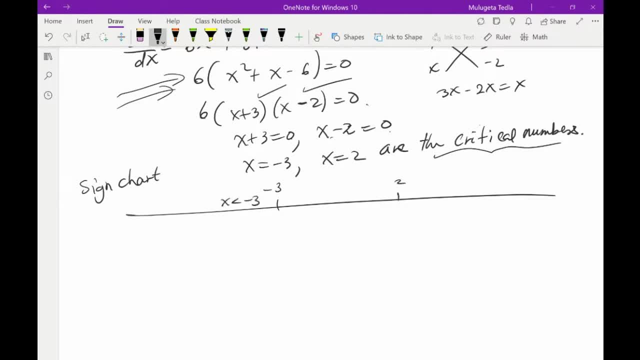 2 as a boundary line. so any numbers below negative 3 and num the, the number set between negative 3 and 2, which we write normally in math like that: any number between negative 3 and 2 is negative. 3 less than x, less than 2 and any number beyond 2 is that. so therefore, the, the, uh well, 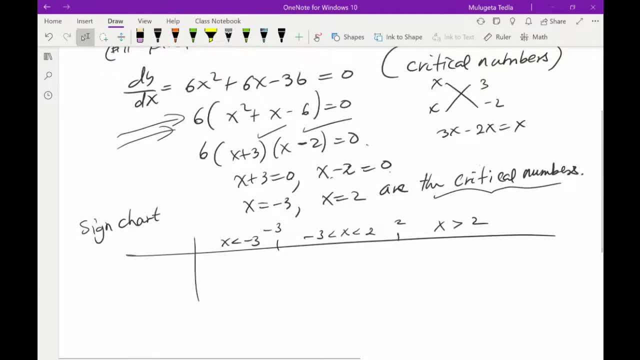 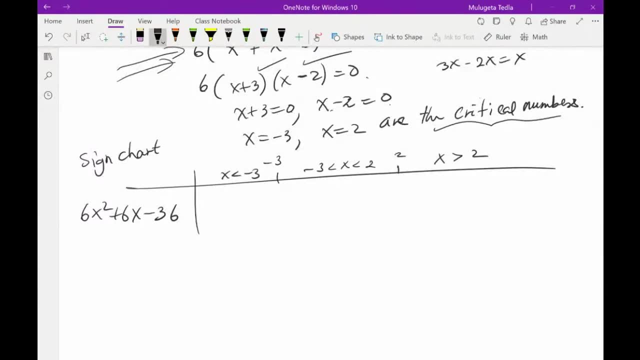 yeah, the, the derivative which is 6 x squared plus 6x x minus 36. you can take a value here in between less than negative 3, say negative 4. plug negative 4 here 6 times 16. uh, minus 24 minus 36. so 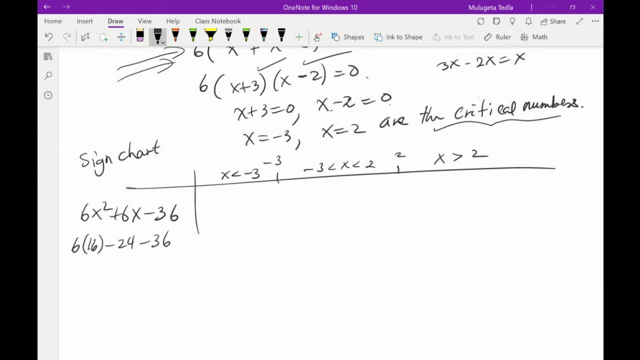 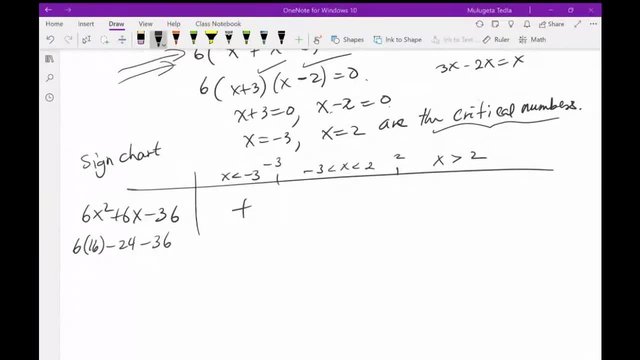 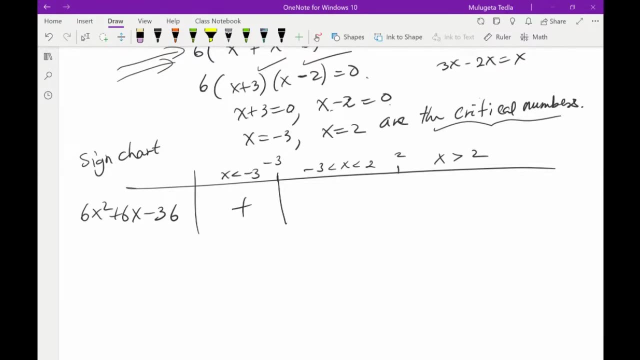 6 times 16 is 96 minus 24 minus 36, it's positive, right, so you get the same answer: positive. thank you, visa. and then than, and then we're going to check a number in between negative 3 and 2. it's 0 is better. 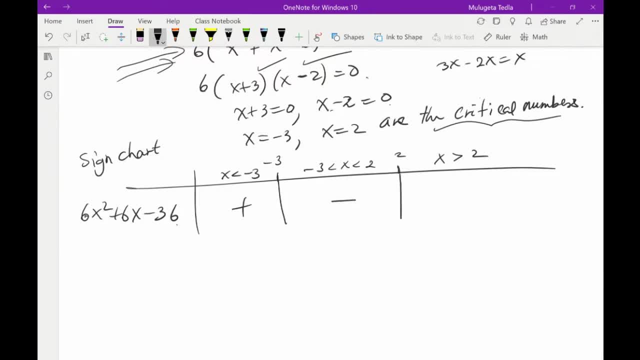 i use 0, 0, 0, negative 36, so it's negative. so at x greater than 2, it can plug three, so it is positive. 3 squared is 9 times 6 plus 6 times 3. it's way beyond negative 36. 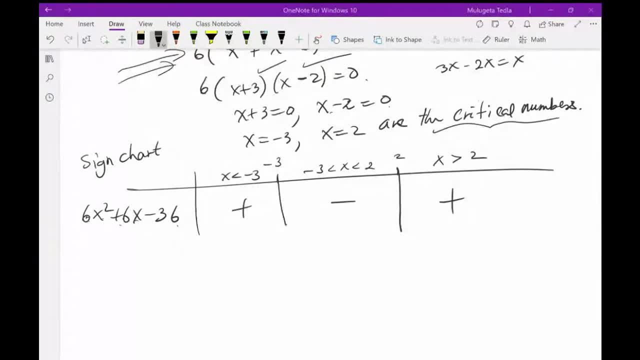 so it's positive, right? uh, sir, i have one question: whenever we get the first sign and then the, the, the rest of the signs, they will be alternating, right, because we are. yes. yes, unfortunately, there are times where you have negative and negative or positive and positive, even between the point. 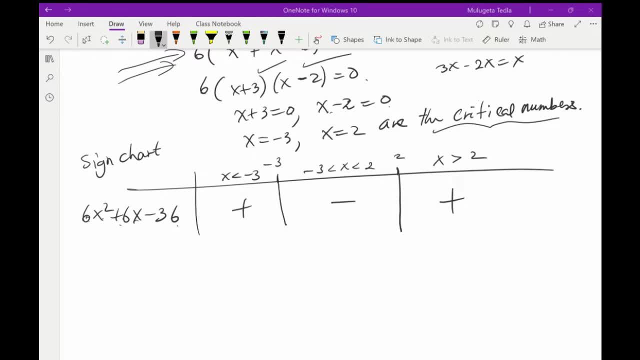 between the reflection point and the turn, the, the maximum minimum point is the same, then the sign dot doesn't change. so there are very rare cases that we cannot just say, oh, plus minus, plus, or plus minus, plus, minus. technically every good graph should be like that. they understand, uh, or some. there are things that have had signs they for, even though they. 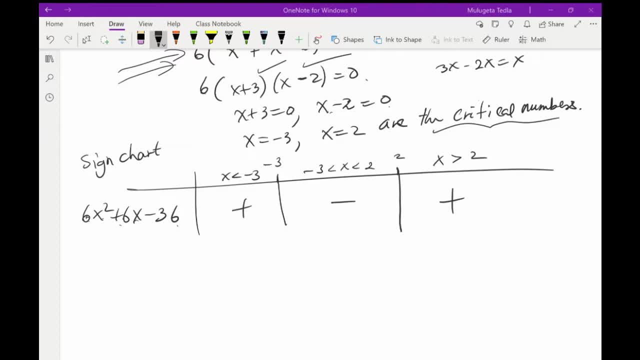 are passing a critical number. uh, if that critical number happens to be, uh, an inflection point which we're going to discuss, there is a chance that the sign doesn't change because of that. can we have an example like that so we can like grasp, i really don't remember, but 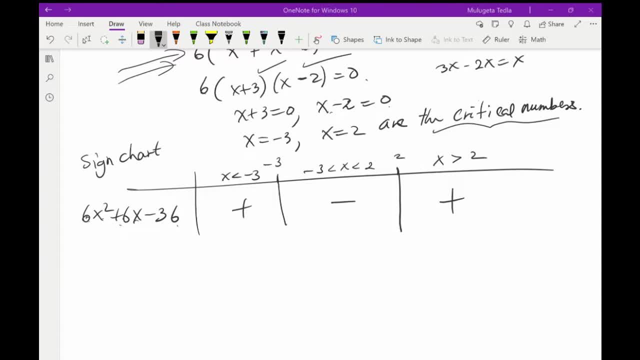 i have done it from experience, i tell you, thank you, yeah, i remember i done it and then that was. there was no sign change because of the nature of the critical number, especially is a inflection point. but uh, for all graphs, normal graphs, this is right. what you say it is right. there is a pattern. 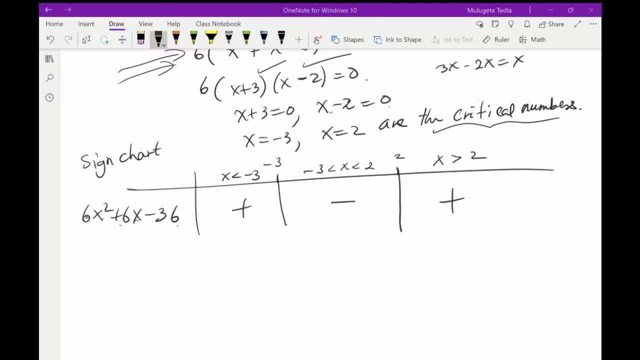 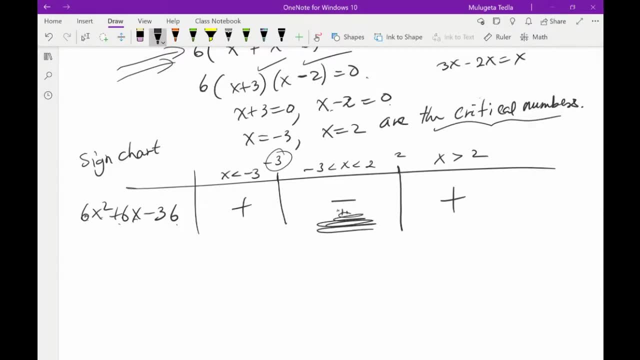 it, there will be a positive number on your first interval. you are logic a yes, it is a yes, here one. Similarly, you change the position, however, you do it in a curve. So here, if next interval, this world, is positive, then if this number three is a critical number, if this number three is a critical number, 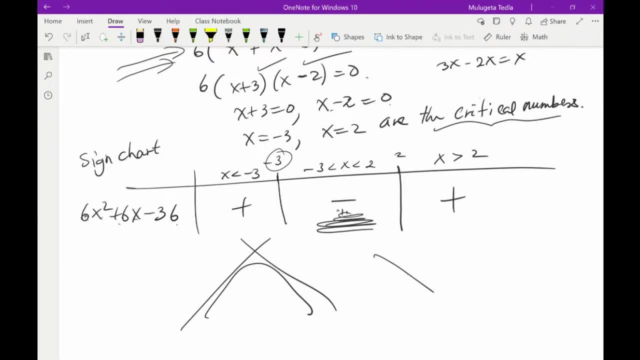 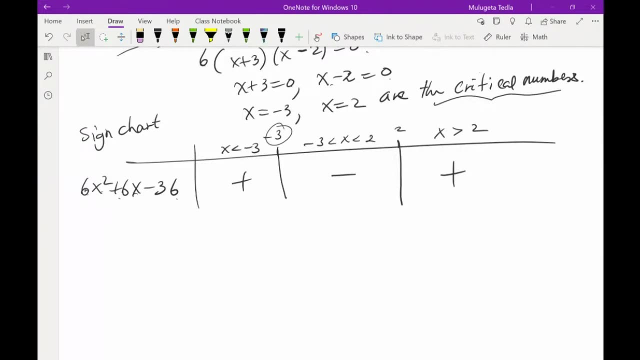 definitely this is going to be negative. We got a change sign. that's what we're saying. So the slope changes from positive to negative or the slope changes from negative to positive have to find this. yes, you're right. yes, the only case- very rare case, it never happens- is what we. 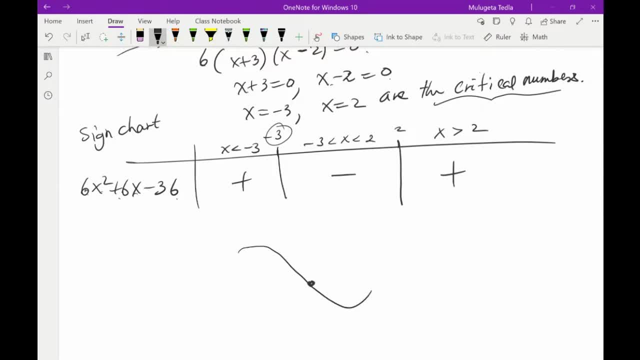 have what we're gonna say. this is called inflection point. so if you have x, if there is a graph like that, you know. so this point is called a critical number, this point where the graph was at a tendency of going down, but at that point it it behaves like going up. the graph wanted to be going. 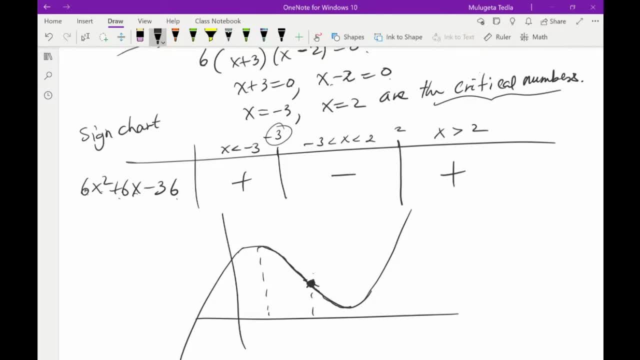 up from that point. that point is called inflection point. that is what the number 15- uh, strawberry asked me to do- is talking about. we haven't discussed that yet, so we will discuss after this example. okay, okay, if, if that, if that is, that point and that point are the same point, this plus minus. 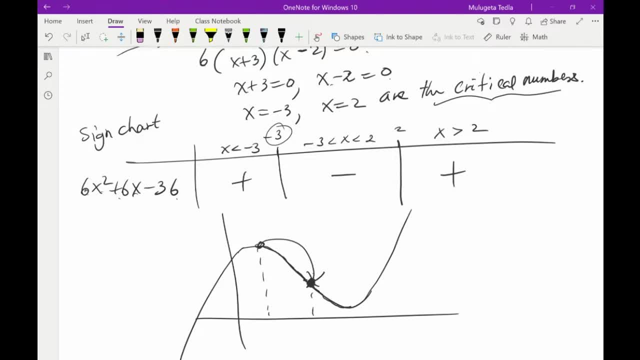 doesn't, doesn't show, and that's very complex, like i mean. that is very rare, it doesn't happen, but it is. as a math person i would say i don't want to say yes, it's always like this, you understand, with some there is even i have seen one where it doesn't follow the pattern. so 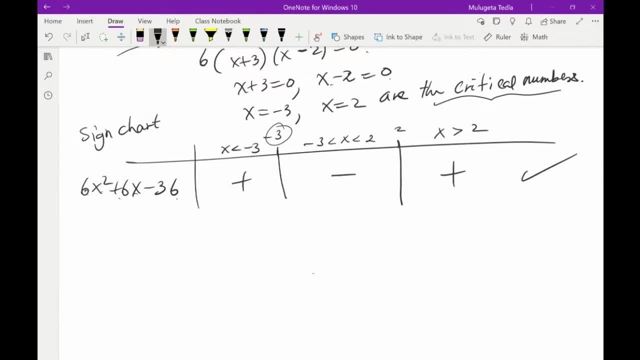 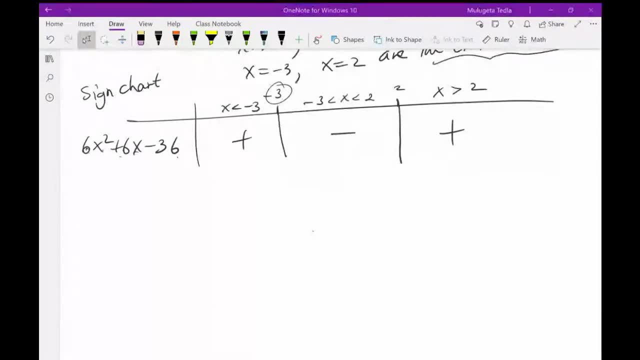 i would say: be careful. but most of the time it is this pattern, right? okay, so you know. uh, class everybody. what he is talking about is like once you get the first interval as one sign plus or minus, he can generate the other intervals without even checking. you know, i i wouldn't take a risk, but i, from all my experience, 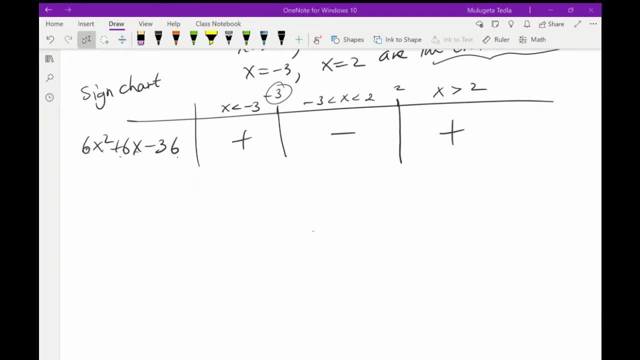 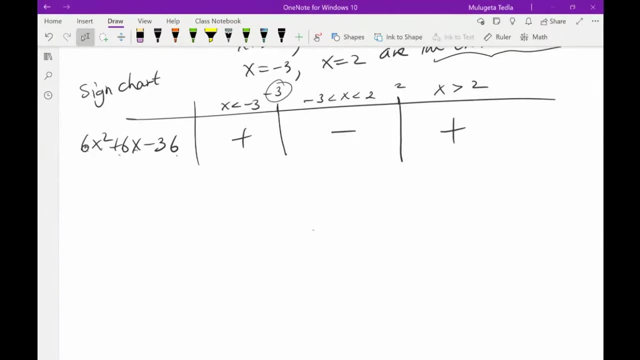 it's that pattern, he's right, he's right. so, uh, when the, the problem would have been if i had plus the first and then i got plus on the second. then there is, uh, a sort of or did i make a mistake? you should check it. you know what i mean. but quickly checking is better, i think. 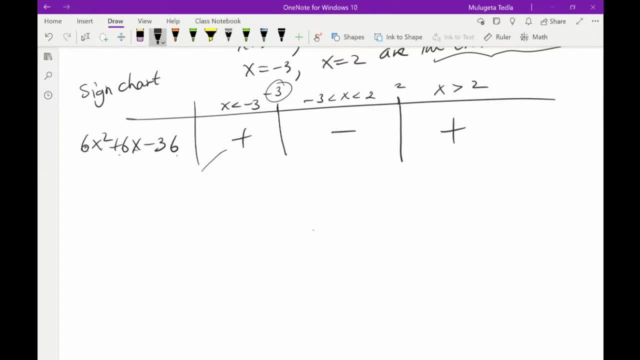 okay, so this is what we got. so, as you know, the slope is positive on this interval. slope is negative on this interval, positive on this interval. so this is the maximum point. this is the minimum point. the interval intervals, now intervals of increasing, which ones are the ones with a positive slope? so it is xx. 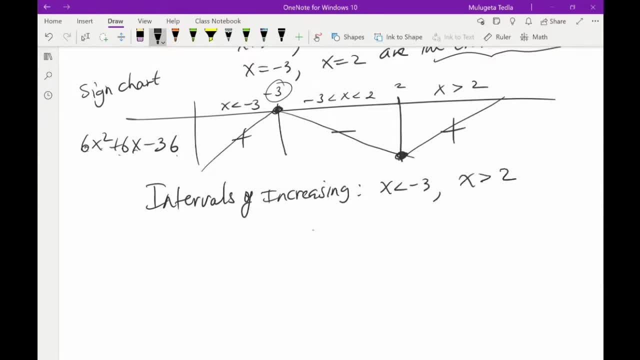 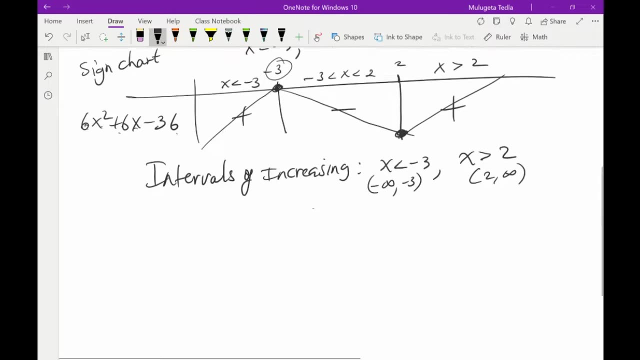 less than negative three. it's increasing. and x greater than two. this the graph is increasing on those two intervals. you can write this as two infinity. you can write this as negative three in infinity. no negative infinity and negative three, all right, so the uh, the interval, uh, 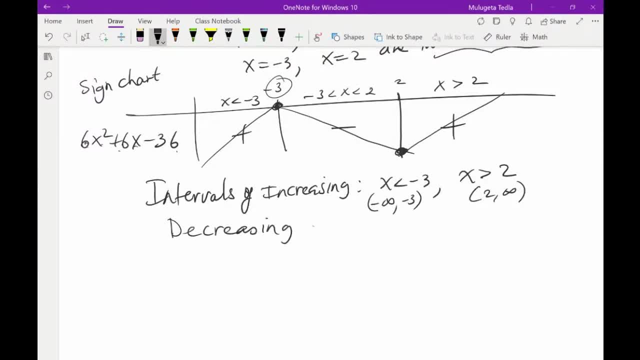 decreasing on the decreasing. the interval of decreasing is only when the slope is negative and it's attained at negative three, less than x, less than two, or in other words, in interval writing, negative three and two. okay, we don't want the critical numbers to be members. you see, this is. 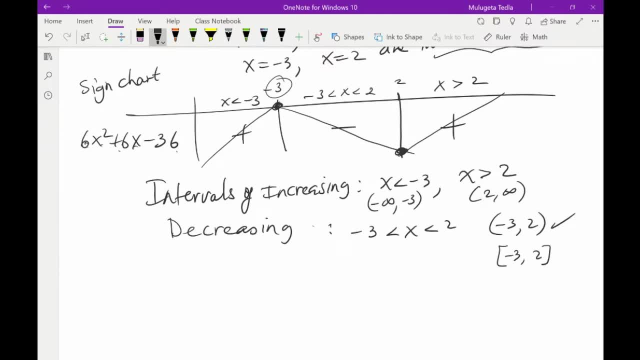 called open interval. this is called close interval. if the two and negative three are part of the interval, we close them. if two is not part of it and three is not negative three is not, it's called open interval because we don't want to include the critical numbers as part of the 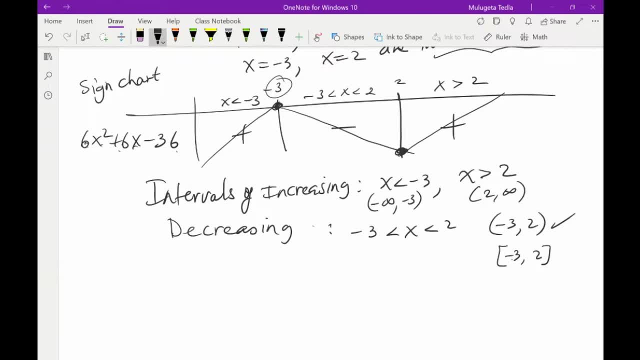 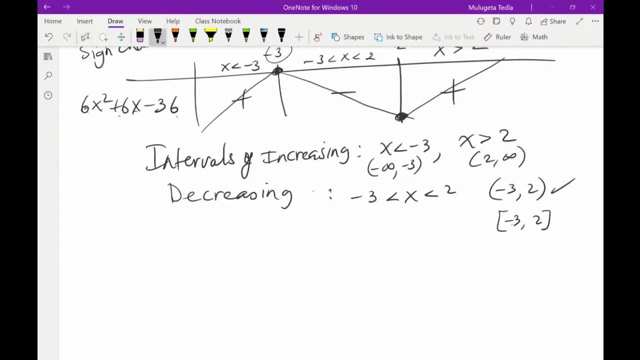 increasing and decreasing intervals, as you can see, because the critical numbers are neither increasing nor decreasing, they are at a zero slope. okay, so therefore, this is number seven. this is the answer for number seven, right from the chart. number 11: the answer is: which ones are local minimum? which are local maximum? of course, uh, at negative three. 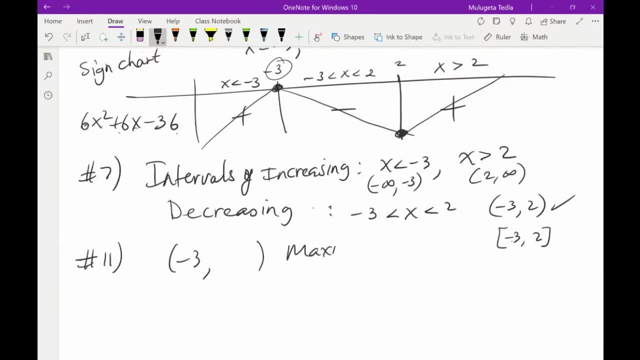 it's maximum, right maximum. but i still have to find y at, uh, positive two. it's minimum, as you can see from here, because when passing positive two from left to right, the slope changes from minus two plus. so that is a first derivative test, right, first derivative test. first derivative test. 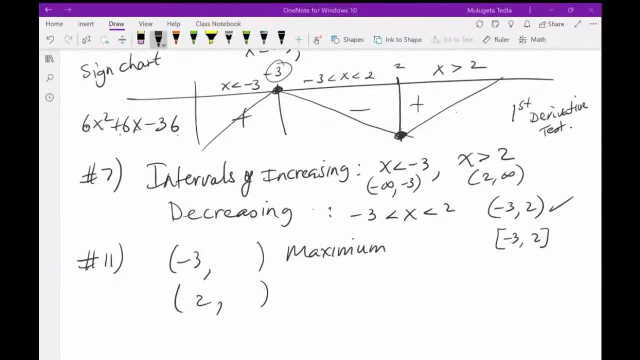 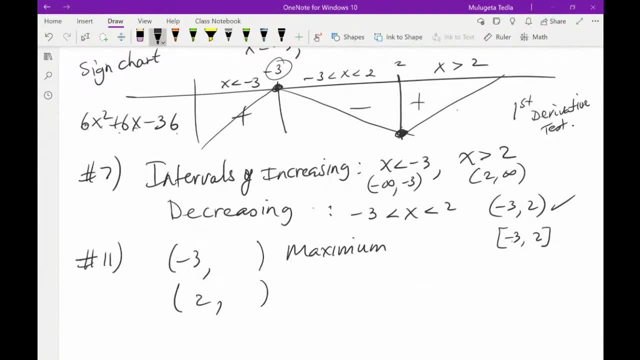 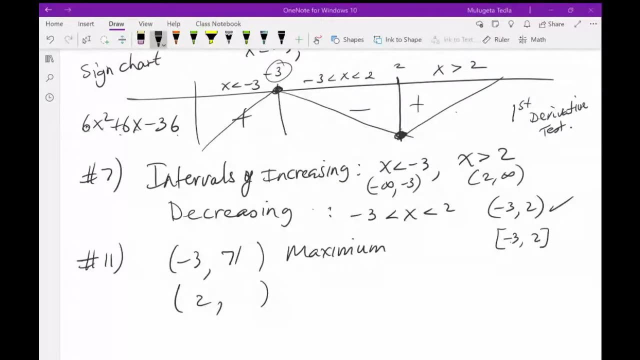 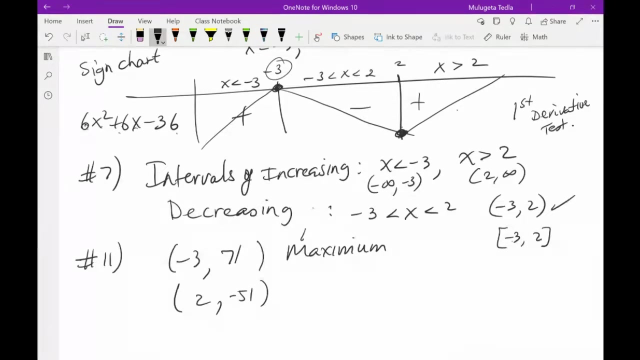 left to right. and last derivative test. all right, thank you was. him has calculated: it's 71 for the negative three and then for a positive two. it's negative 54, negative 54.. so these are the two. this is maximum local maximum local maximum point. 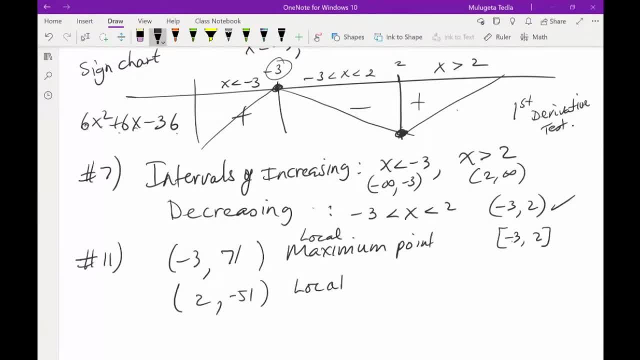 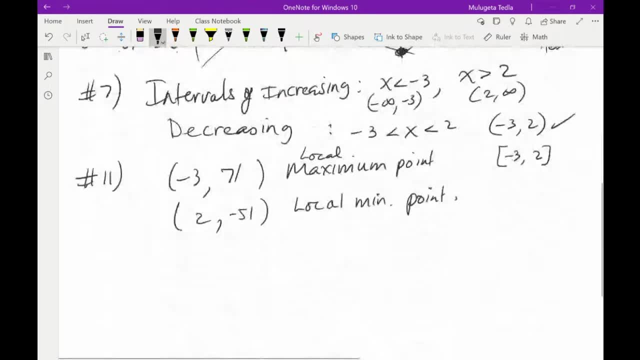 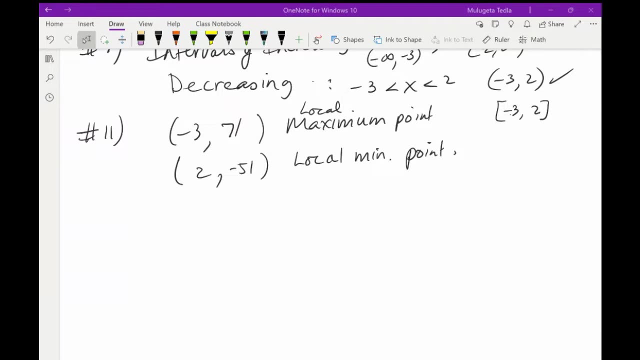 this is the local maximum minimum point. right, this is number 11. that's that's why they are asking: okay, is it okay what i have done? uh, who asked me those questions 7 in 11 is actually eric. eric, did you follow me? uh, hopefully, 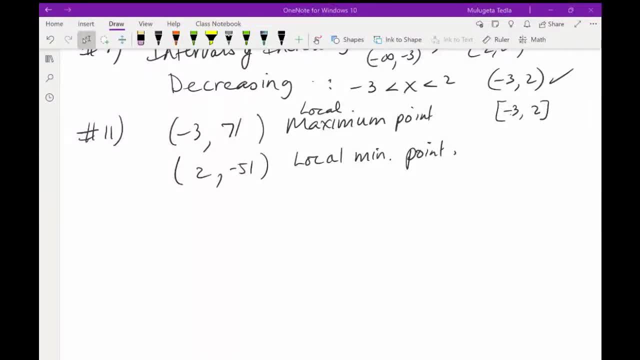 or you have any questions. uh, follow-up questions. is it minus 54? okay, i will do that. yeah, was there any other question? then, on number seven, when you did the points of uh or the increasing, it kind of looks like that's supposed to be a y value, but it's not. 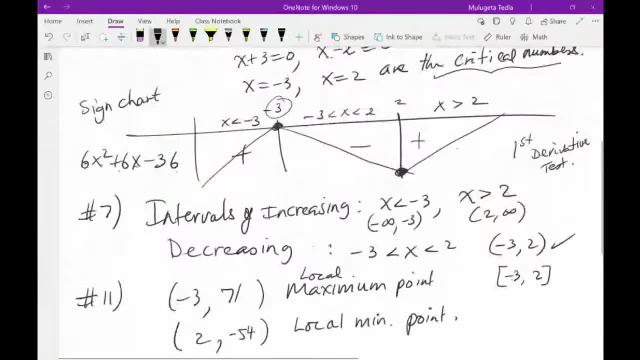 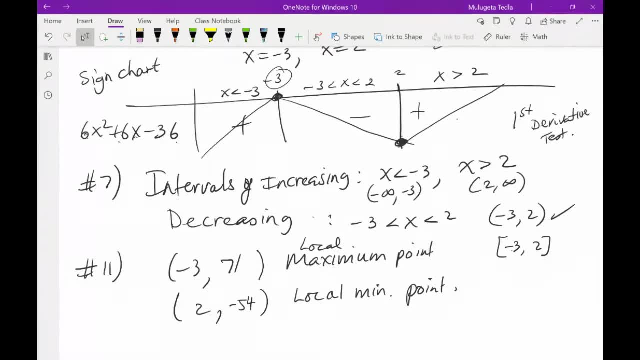 right. is there a better way of writing that which one, which one um say: decreasing, negative, 3 comma 2, decreasing, yeah, the interval of my writing: negative 3, less than x, less than, uh, positive 2, or the interval negative 3, 2 comma 2, in brackets, uh, could you repeat the question? yeah, like the brackets that. 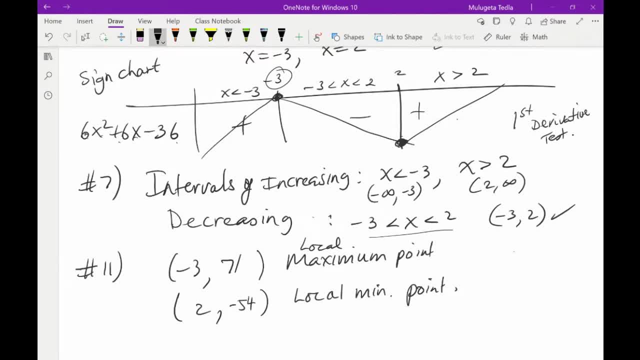 kind of looks like it's a y value, but it's not right. you're just referring to the x. oh yeah, yeah, you mean this one. okay, very good, okay, because this is not a coordinate point, this is an interval. we call it so interval. you're right, if you. if you consider this a point, yes, it is x and y component. i'm. 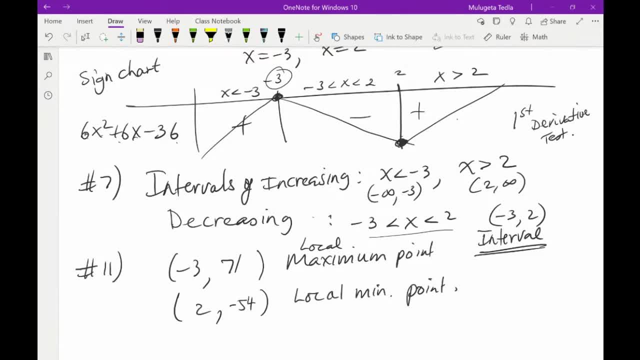 not referring to to. i know i should explain that. so this is interval. this ordered pair could represent two things. if you're talking about intervals, like what we did, intervals here, then it is. it is not the y value and the x value. no, if this, this is a point. 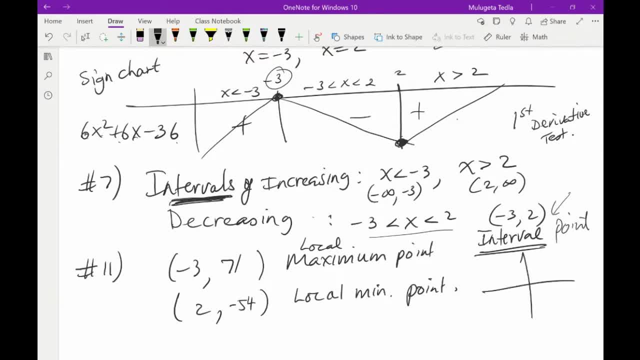 then it is. it is a point on the plane, on the point on the plane. negative 3 is for x and 2 is for y. so this is a point. you know what i mean. so it's an alternative way of representing enter intervals. if you don't like it, stick with with this, okay. 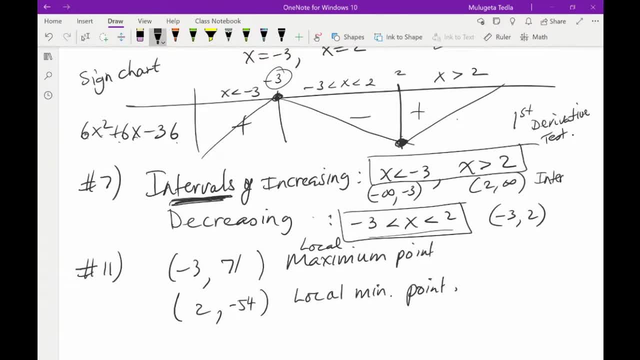 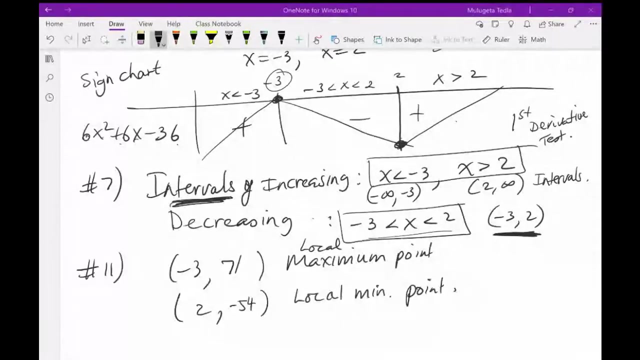 okay, thanks for explaining. i hope you understand the answer. yeah, i think the word interval should be accompanied by this kind of writing: okay, to avoid confusion. is that what you mean? the? the confusion was there because it looked like an ordered pair. is that that what i sensed? yeah, thanks, yeah, yeah, eric. 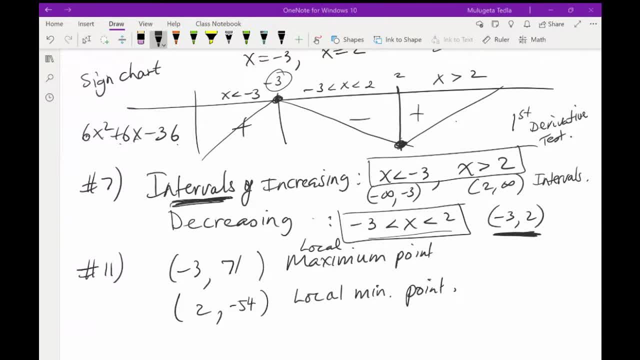 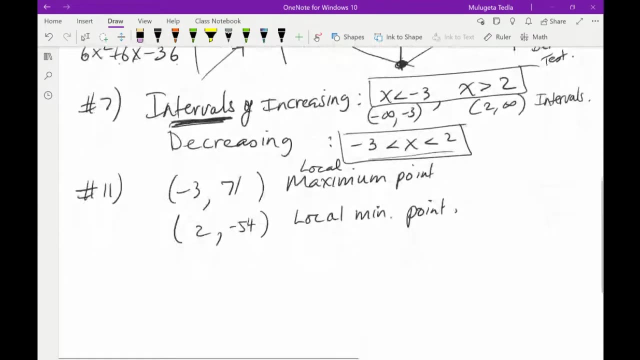 so yeah, i should mention interval or something, but when you put it in an ordered pair of uh numbers separated by coma, you're right: the first coordinate is x, the second coordinate is y, but if it's confusing you should avoid it. yeah, so these are like the coordinate points. so 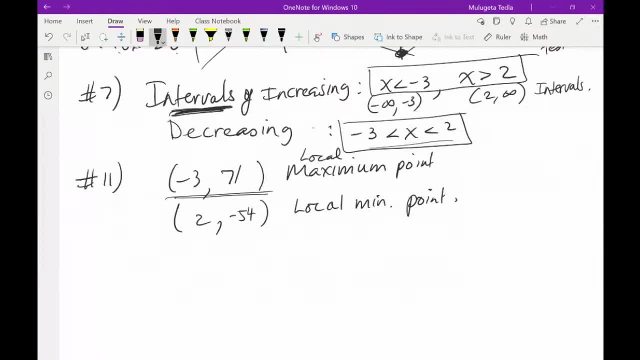 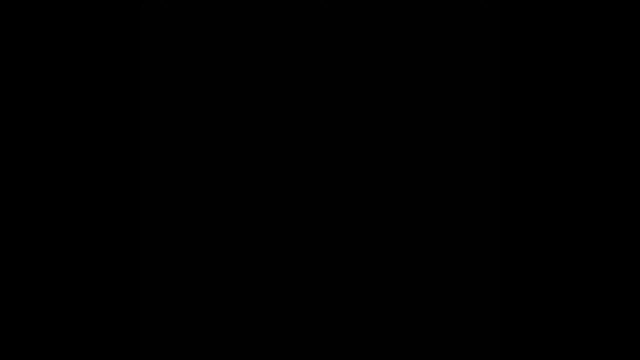 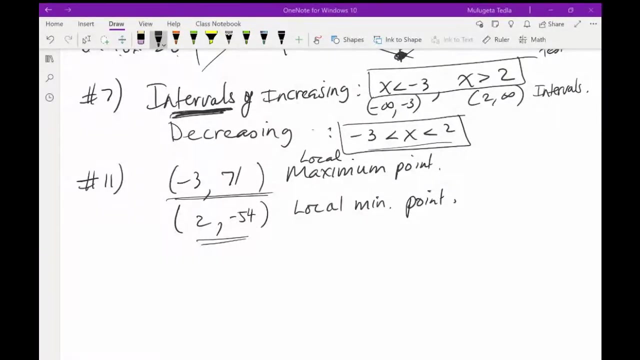 is uh negative. 371 is a local, local maximum point and then negative 54, yeah 2 and negative 54 is a local minimum point. okay, uh. so anybody with uh any uh follow-up question on those? are you okay with this so far? finding the increasing decreasing intervals, finding the 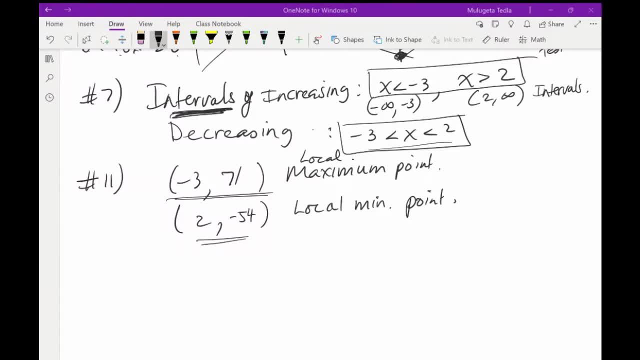 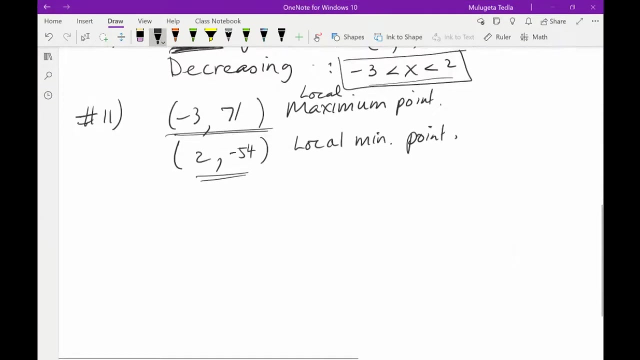 uh, local maximum and local minimum, because i'll i'll ask you on the test. 100. okay, you gotta ask me otherwise. oh, sivan, you have. uh, was it 2 and negative 18? uh, sivan, did we make mistake somewhere? yeah, sure, so it's stated that the next last number is negative. 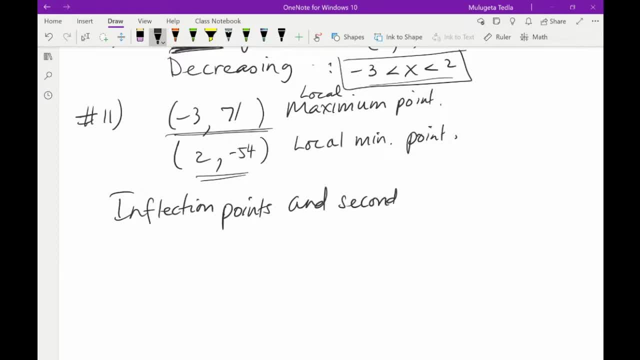 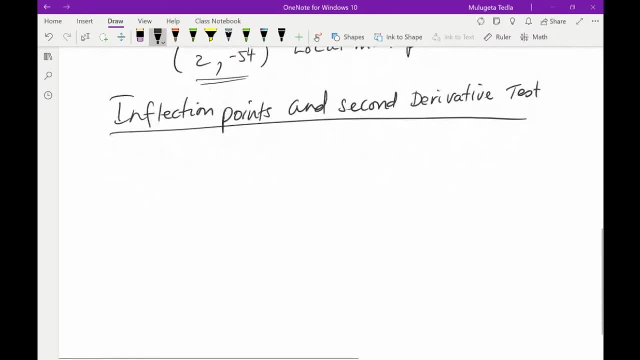 And second derivative test And second derivative test. So what is an inflection point? An inflection point actually is a point where the point, the graph, changes from concave up to concave down or vice versa. No, So I think that's good enough. An inflection point is an inflection point is a point where the curve changes from being concave up to concave down. 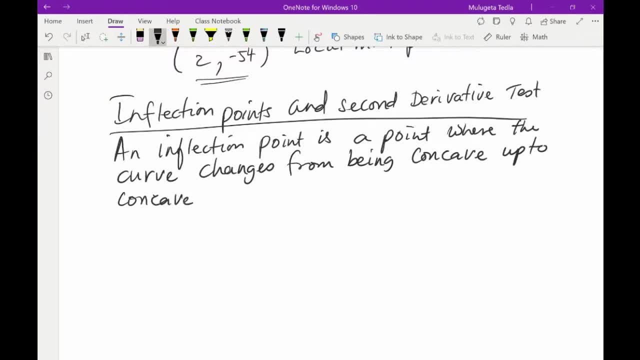 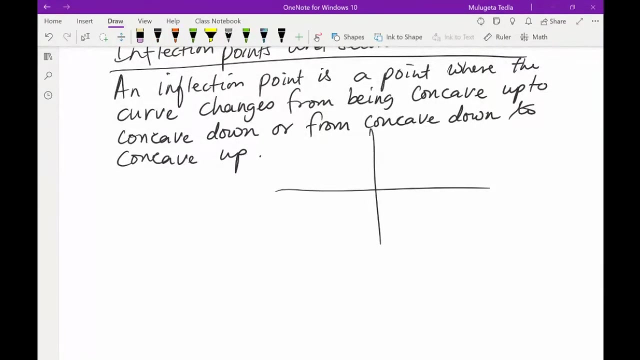 To concave down, Or from concave down to concave up, So as an example of a drawing. So if you have like that, If you have like that, So this, this point, let me call it X1.. Why, Why am I interested in this point? Let me call it X2.. 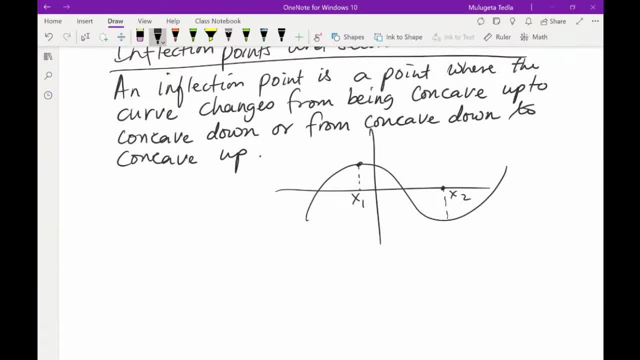 I am interested on those two because they are peak points. They are local maxima and local minimum and they are called what? Note that X1 and X2 are called what? What did we call them? They were called critical numbers. What are critical numbers? 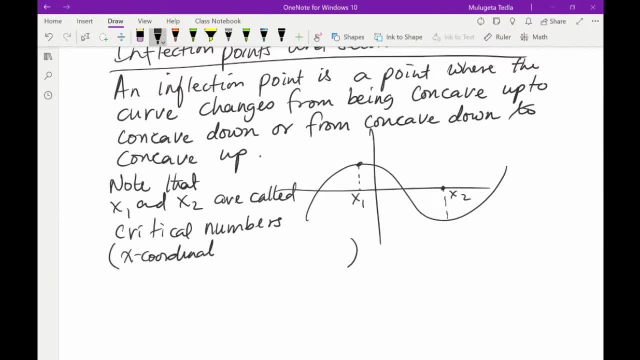 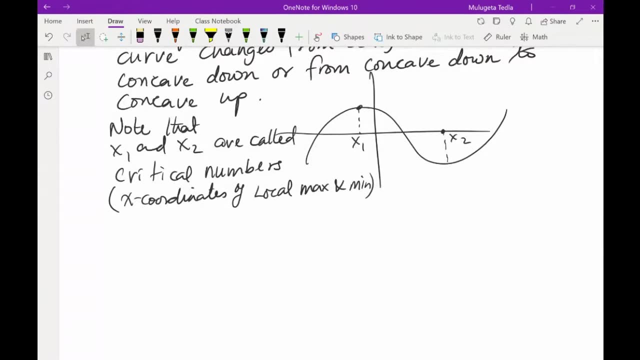 The X coordinates of local maximum and local minimum and minimum. These are what we said. We've been doing that the last two classes, And now this is that number two. But this point, which is halfway Here, maybe here You know, here this point, this point, let me call it X. 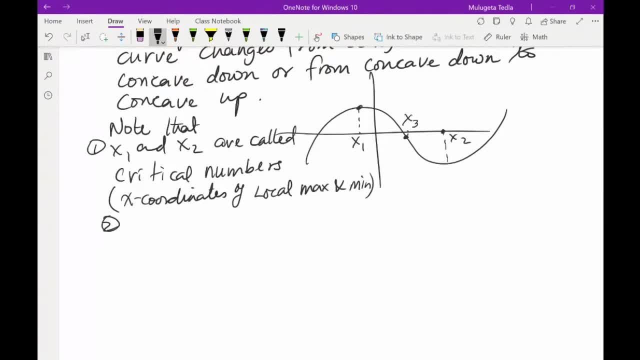 My numbering was not X3. OK, X3 is an inflection point. An inflection point, you know, you can see that, because the tendency of the curve to go down, Right to go down, Right to go down, is up to that point and then it feels like it's trying to turn up. 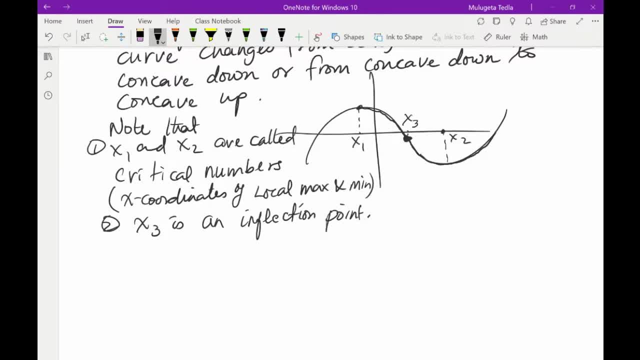 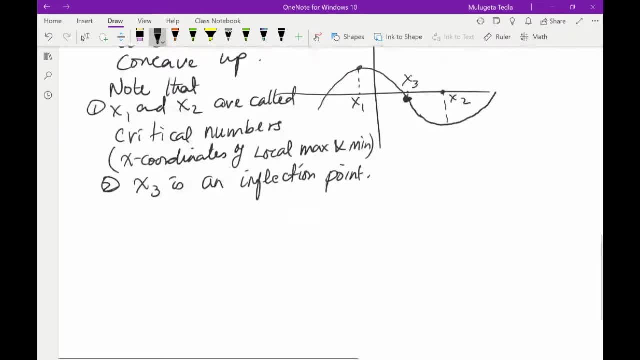 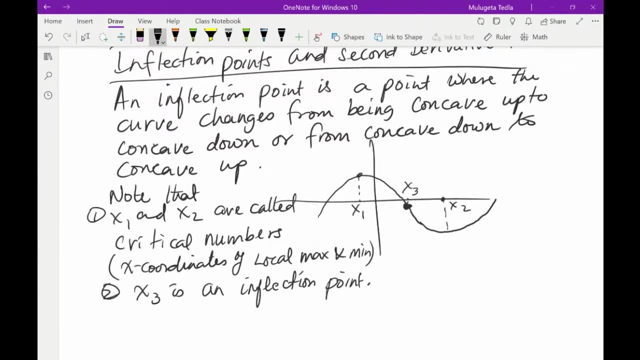 word. so that point is inflection point and it is very easily found in math. in mathematics we can find. so what did? how did i define it? an inflection point is a point where the curve changes from being concave up. it was concave up, here it's concave down, it changed. 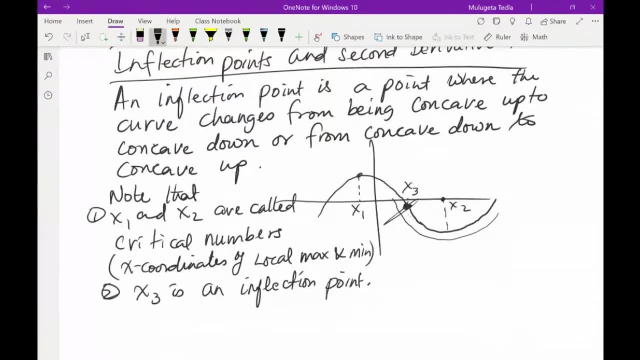 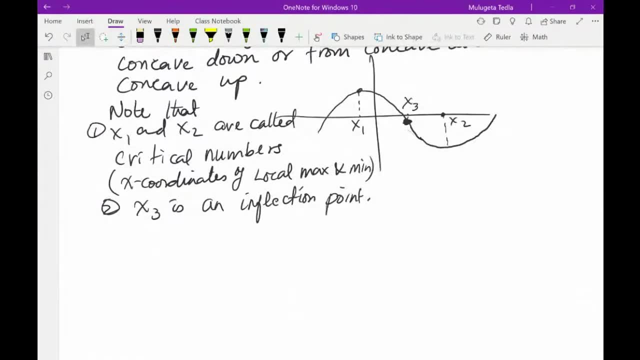 from the tendency of concave up to concave down at this, at this point. so that is inflection point, and vice versa. okay, so x3 is an inflection point, but x1 and x2 are turning points, they are maximum and minimum points. i mean x coordinates of those points. 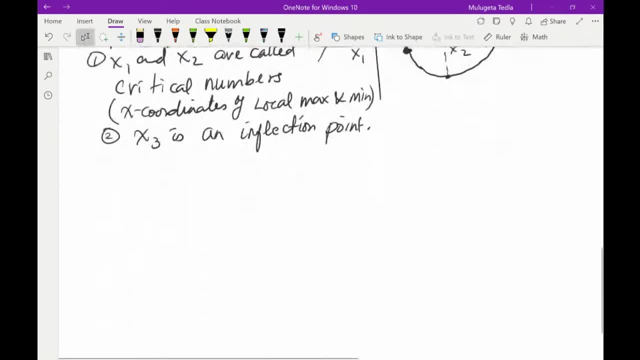 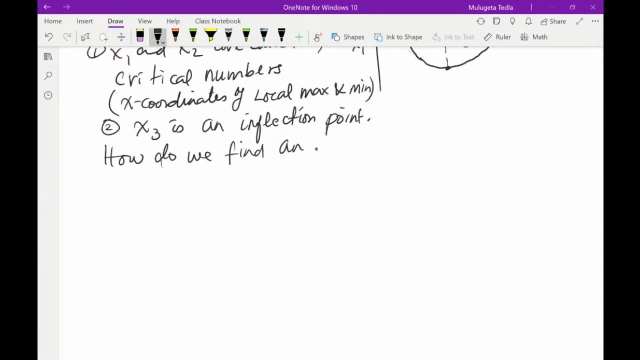 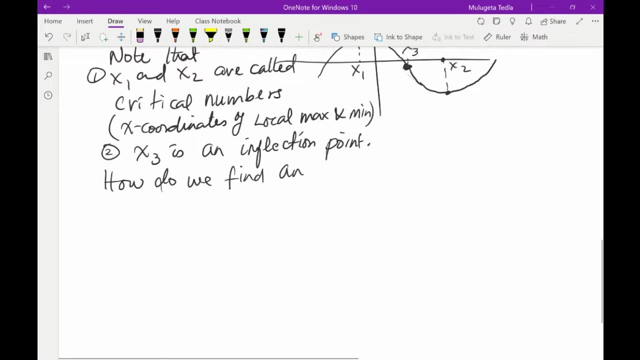 okay, so, uh, how do you find an inflection point? how do we find an inflection point? uh, could you do you remember? how did we find a critical number? how did we? how do we find an inflection point? right, i just want to ask you: how did i find the critical number? 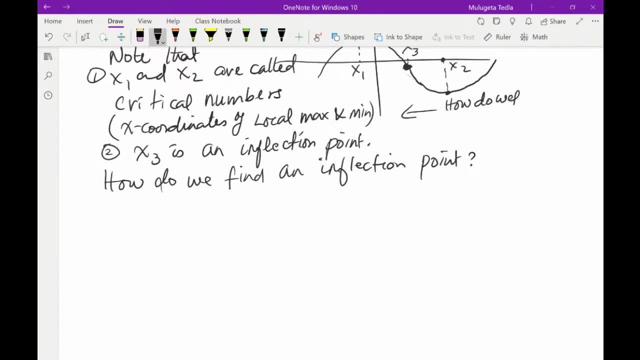 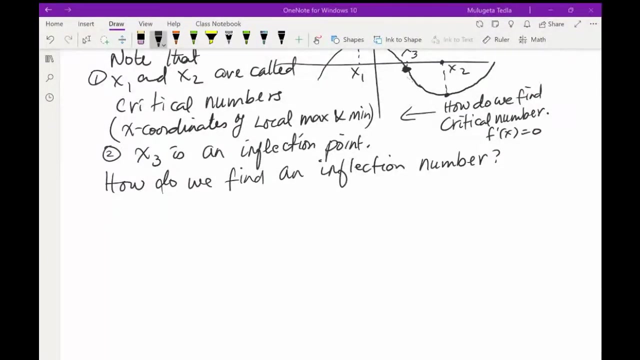 how did we, how did do we find that? yes, how do we find a critical number? f prime of x equals zero. now, how do we find inflection point or inflation number? let me call it, because the point will be: uh, yeah, maybe i have an answer. second, there will be equal to zero. okay. 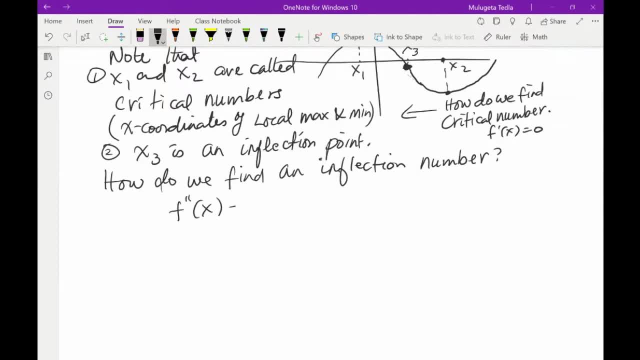 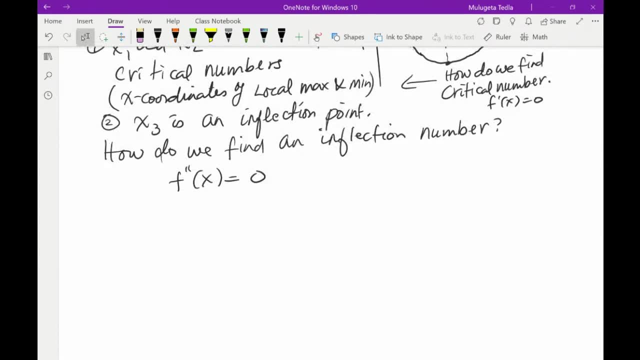 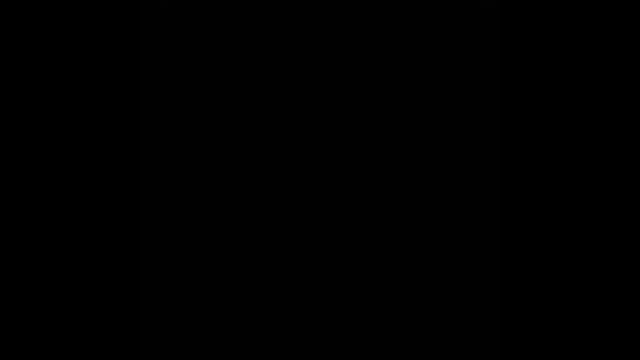 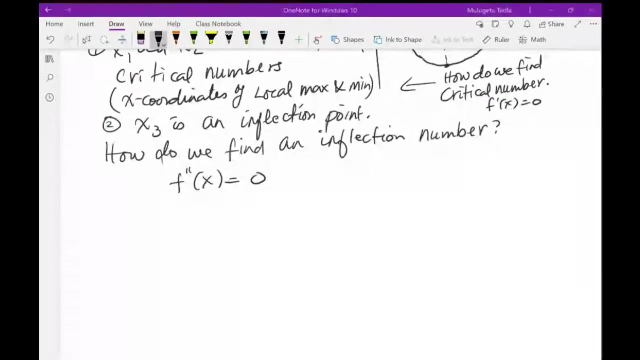 second derivative f, double prime of x, equals zero. right, that's exactly what it is. uh, can you mute yourself? uh, however probably, or i can mute the whole class, otherwise. okay, thank you all. right, i don't know why this is happening. so, second derivative equal to zero. 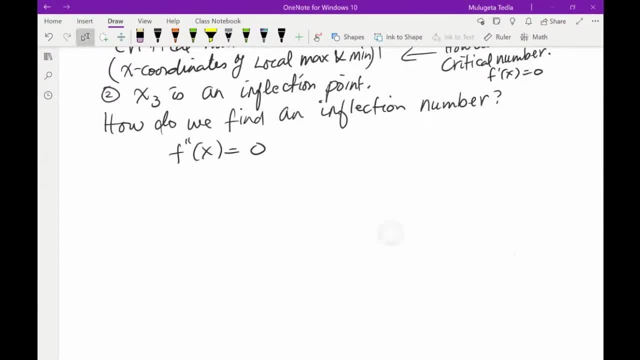 is actually the way to find the inflection point and solve for x that x will be inflection point. okay, that is one thing. now the, the uh. there is another test, what we call uh, second derivative test, second derivative test. this is an alternative way of the first derivative test. how do we find a critical number? if it is? 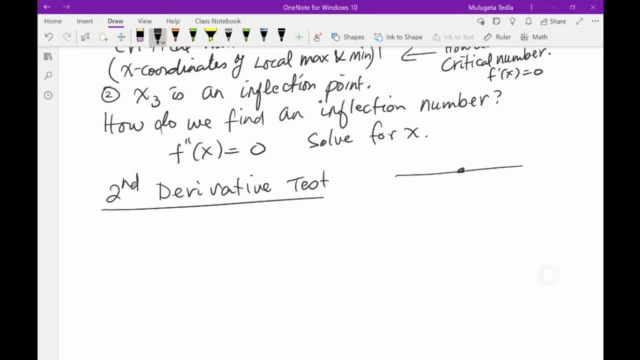 first derivative is e. very easy, it's more like using side chart. we said: if this is a critical number anything below x less than c, if the slope changes from plus to minus and this is x greater than c, then if it's plus to minus, then c is maximum. we said. 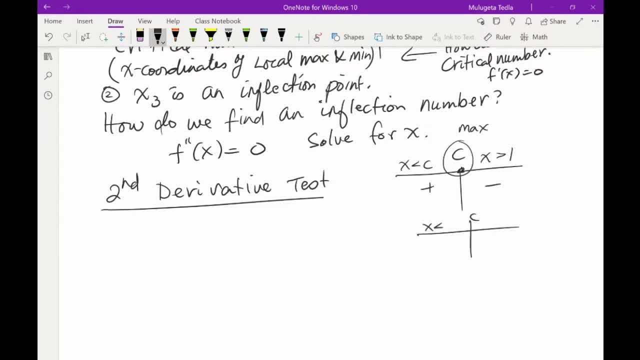 if it's a critical number here, x is less than c and x greater than c. the slope changes from this is dy by dx. this is dy by dx. if the dy by dx changes from negative to plus, then it's going down and up. so it's minimum point, this, this critical number. 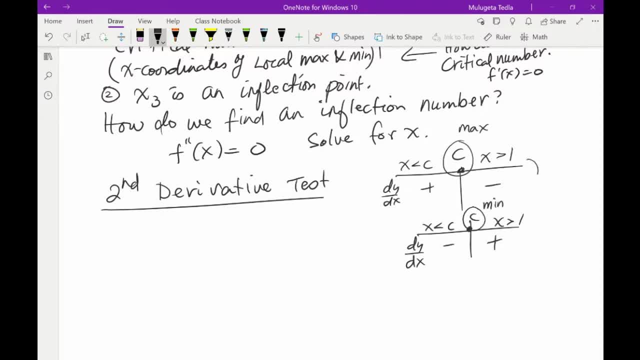 is a minimum point. that's why we- this is what first derivative test, if you remember. that's why we did last class. okay, secondary test is another alternative way of testing. uh, okay, another another way of testing: local minimum and maximum points. uh, is the secondary test. it's very easy and it's very effective for polynomial functions. 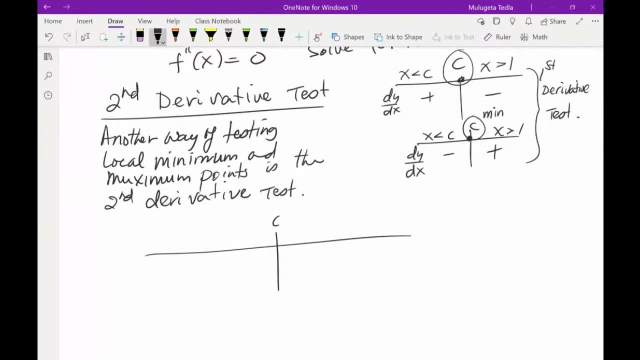 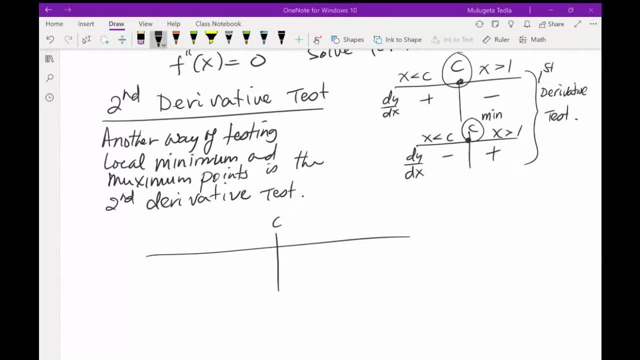 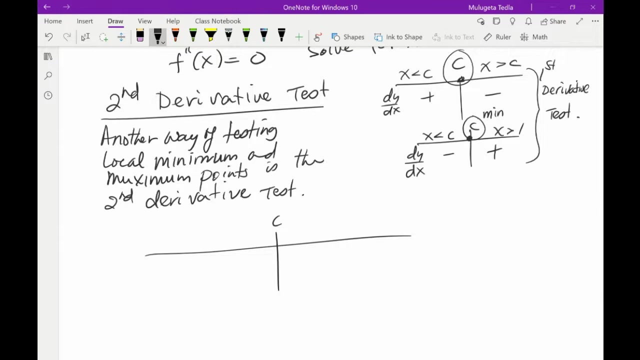 so what it does is, if you have a critical number- critical number now, unlike some other equations, you might help us to solve that. was is Similarly shown on the first line of this problem. we actually write a low Fahrenheit down here, so you show your nearest derivative, the solarStopela. 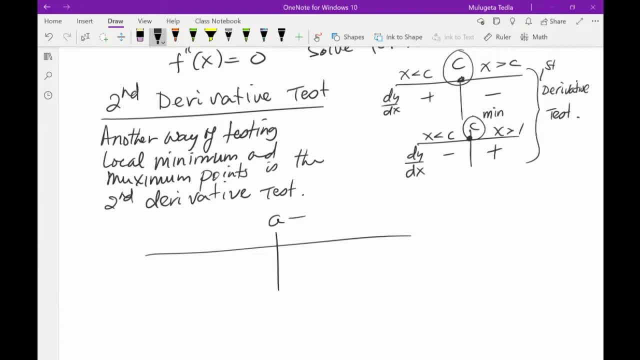 so then it's going to be the second derivative. I will see from the first line. we see the lower Patriot of the derivative as our the in and the left tamer on this unit, so these два variants were same. we are going to see what is going on in terms of comes down here and again the 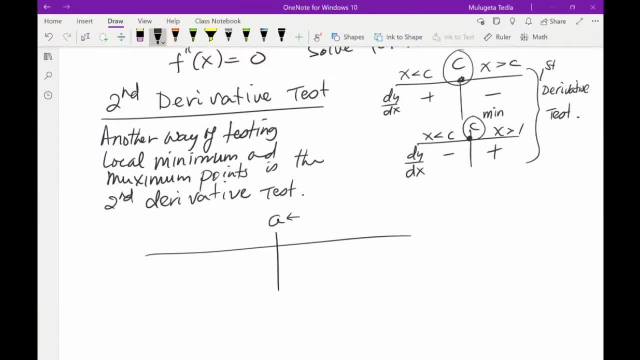 testing because it's not a minimum or maximum point. this is critical number. how do we find it? we find it by f prime of a equal to zero, not f double prime. we find f prime of a is equal to zero to find a critical number. what is the test? okay, if you find the second derivative. 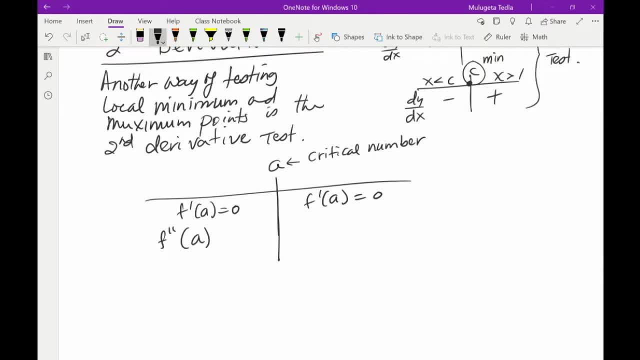 and you plug your critical number into the second derivative if the sign is negative. if the sign of that number is negative, then it's maximum local maximum point. then x equal to a is local x coordinate of local maximum point. or i could say a and some y is a local maximum point. local maximum. 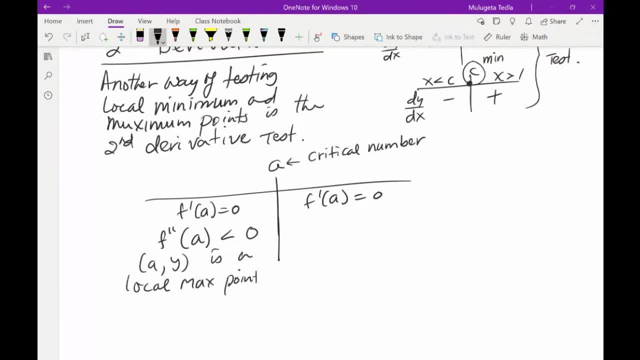 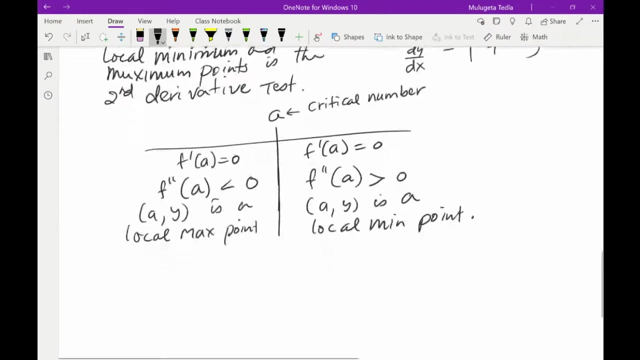 point point. so if f double prime and if you plug it, if you have the second derivative, you plug your critical number and you get a positive sign. then a y is a local minimum point. now i will do number 15, what strawberry asked me to do as a homework for for two. 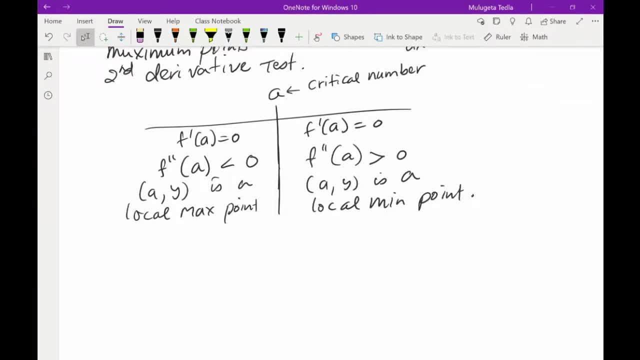 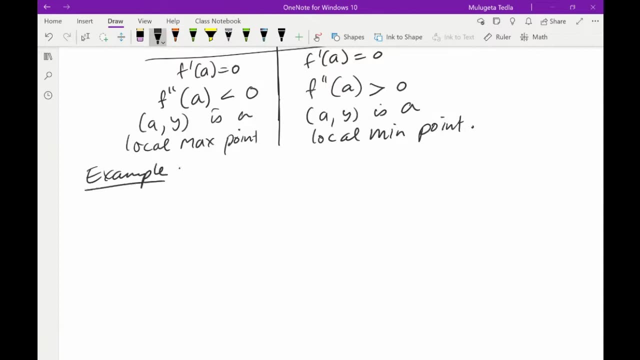 exactly, you know, to justify, or at least to give you a clue what i'm talking about for those two, two concepts. the two concepts are inflection point. and then what is the second derivative test, right? so number 15 example. so we'll do some questions on. uh, sir, should be like the f double prime, a equal to zero. 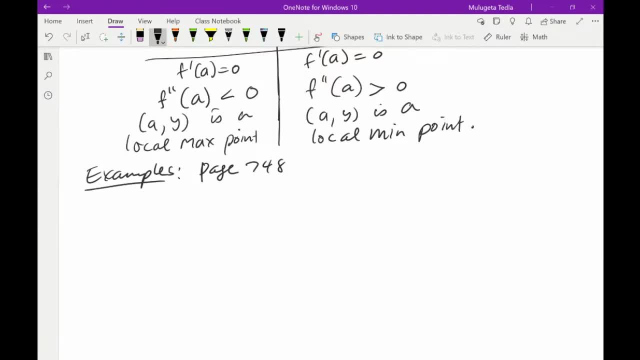 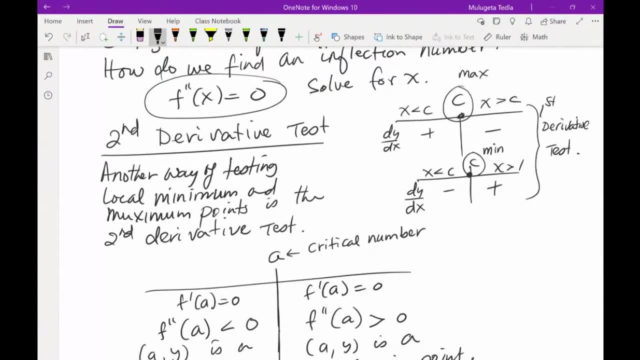 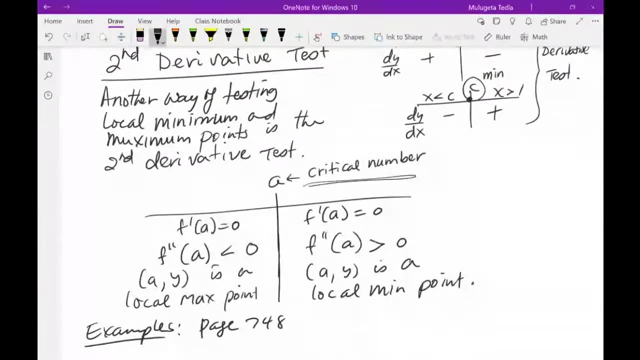 equal zero and no, that is for the critical number for inflection point. to assume that is for inflection point i mean on the chart is: is the? is it for inflection point? the fa equals zero. this is, this is, uh, for critical number. no, the chart is for critical number and the test will be fine. 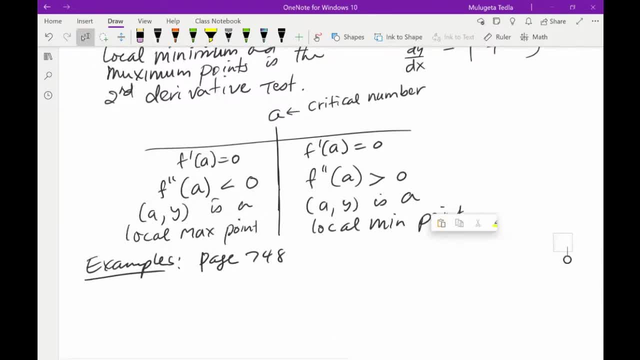 and alternatively we find: yeah, do we find the critical number by equal? I mean for inflection. we find the critical number by equating the second derivative to zero. No, don't Be careful, What we call critical number is only if you use F prime, not F double prime. 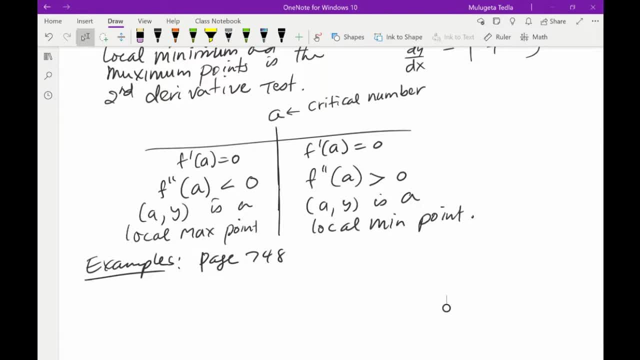 What we call the inflection point is when we use F, double prime. But here, like we use both of them, we put A, Like we are mixing them, A critical number. to emphasize a critical number. I use that Nothing. This has nothing to do with the test. 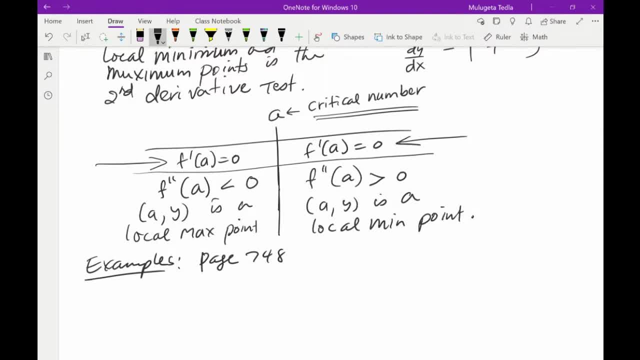 But you know that a critical number, if we call it critical, the derivative, if you plug it on the derivative, it becomes zero. That's what it is. This is a test. And then ask me now: Yeah, OK, And the test we do it like. 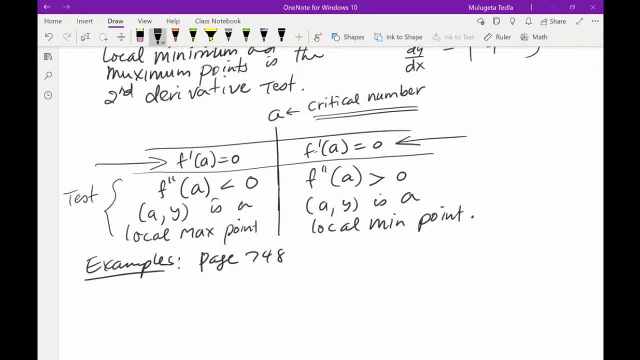 You agree with me. like the critical number for inflection point is different than the first derivative right, Each one of them has its own. So in this case we need also to find another critical number for F. double prime equals zero, right. 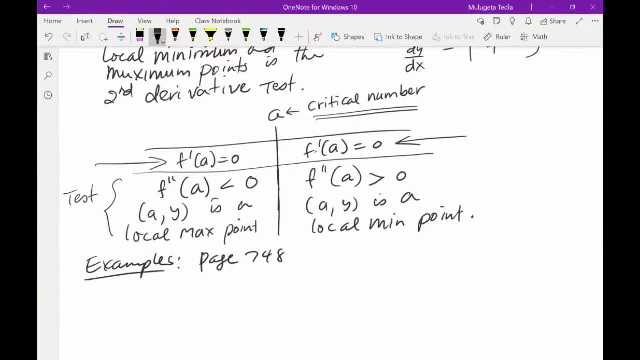 It's another critical number. No, I mean, we don't need it. We are testing the critical number. We don't need F double prime of zero. F double prime of X. Right, It's equal to zero. We don't, unless we are asking for inflection point. 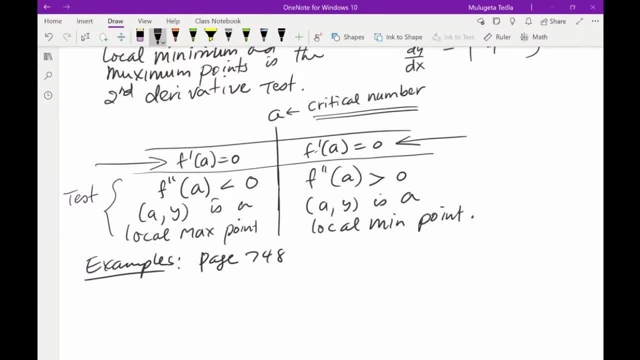 Yeah, This is not for inflection. I thought it's for inflection point. That's why, OK, No, no, It is critical number. We are testing on the second. Oh, second, Oh, OK, OK, Thank you. 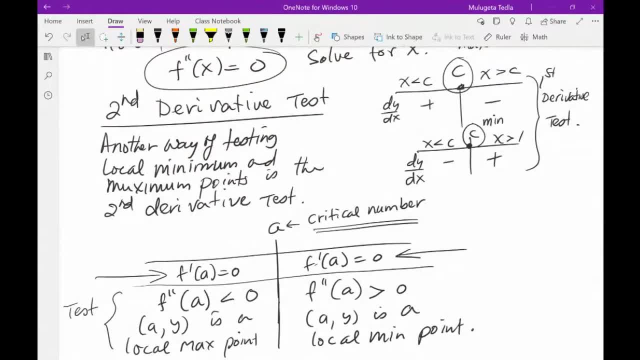 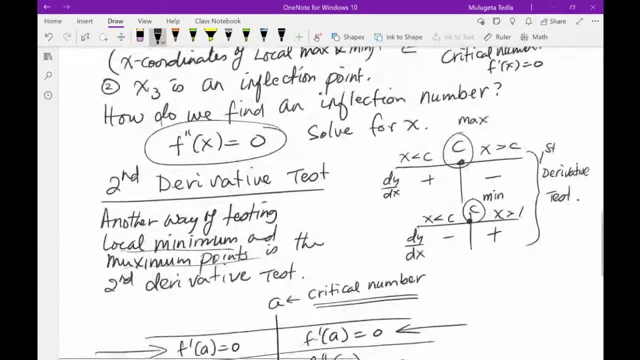 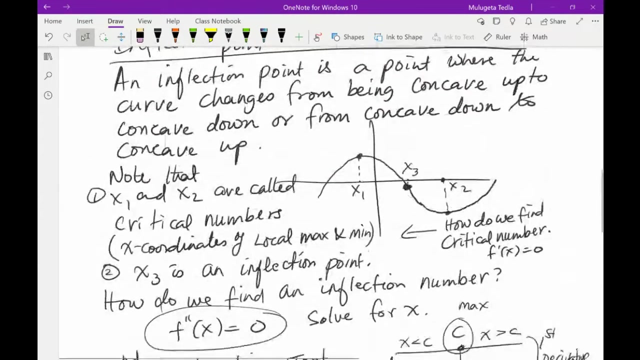 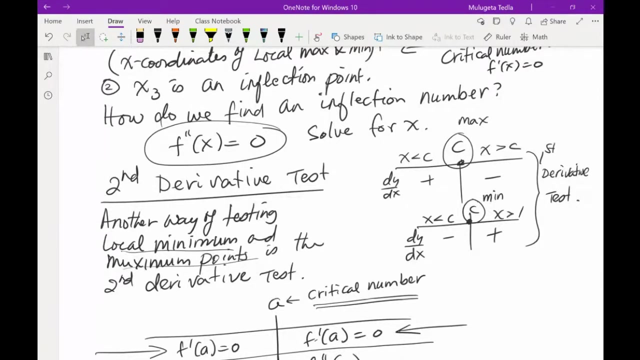 OK, No problem, I want to. I want to emphasize: when you're testing local minimum, local maximum, We only test critical numbers, which is the number we get from the first derivative. I think the category came, unfortunately. I am talking about inflection point and then talk about secondary test. by it kind of senses that it is mixed up, but the secondary has nothing to do with the inflection point. 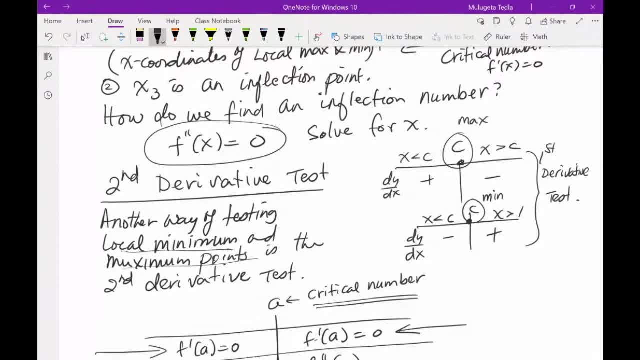 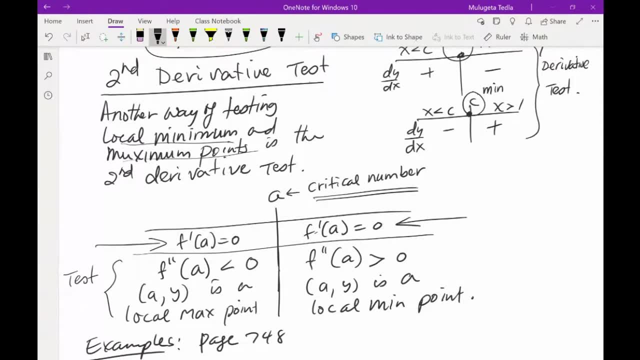 OK, so what I mean is, on the secondary test, I am still testing an alternative way of testing local minima and local maxima. So if I am testing local minima, which one is local min, which one is local max, I am still testing whether the critical number is local minimum or local maximum, not the inflection point. 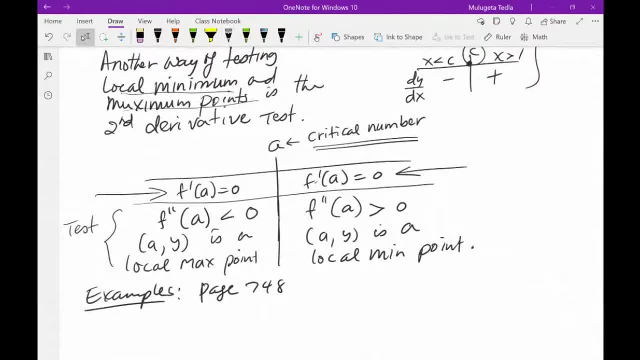 We certainly are not happy about that explanation. No, because there will be too many criteria, Like: the first test is not enough For local maximum. Oh, yeah, yeah, yeah, It's not. it's not enough because more trigonometric functions listen for more trigonometric functions. 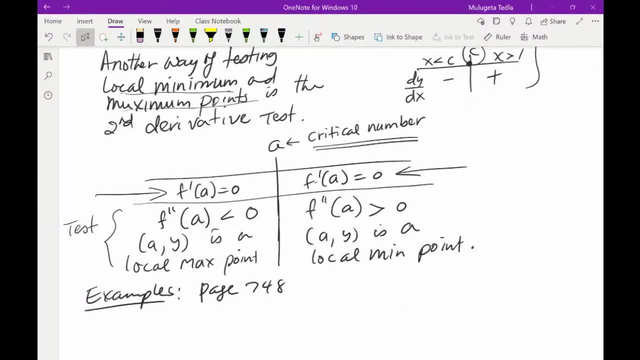 We most of the transcendental when we use transcendental functions like logarithms, exponential functions, trigonometric function we use for us to test because it's very easy to plug numbers in, But for polynomials because it's very easy to find the second derivative. 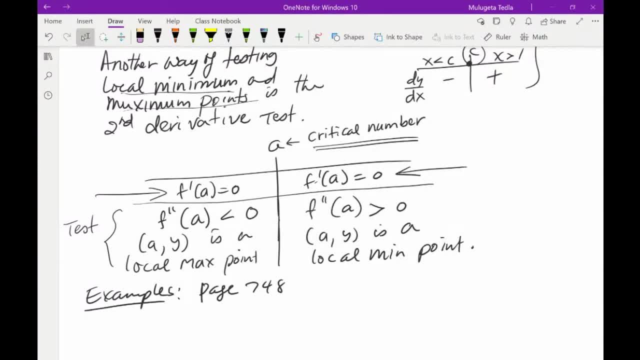 We prefer the second derivative test. They have their own advantages according to the, to the nature of the function you're testing. You understand. So, oh yeah, it's easy. OK, yeah, So the book cover both of the tests. 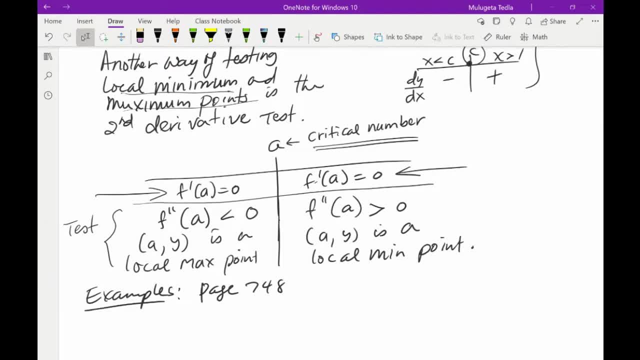 As students, we learn the tests And then when we use them, we use them. It's just the fact that mixing up the inflection point with the testing is not right. That's what I'm trying to say. It might confuse you. 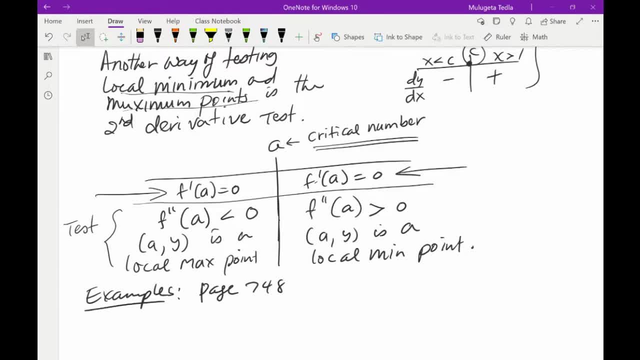 Yeah, The inflection points are simply: you find the second derivative, you let it to zero, you find your inflection point, the X component of the inflection point. Then that business is done. I'm not testing the inflection point. 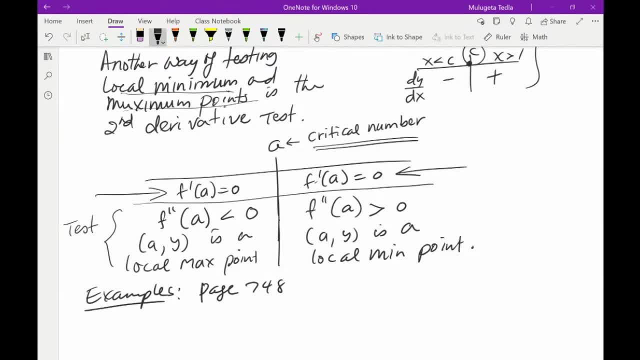 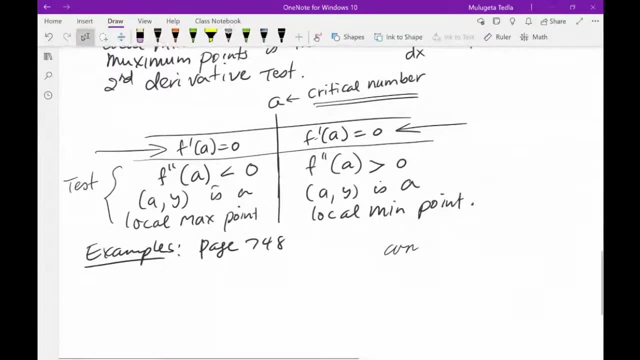 I'm testing the well I will. If you're talking about local, I mean, what do you call concave up, concave down? That is another test. A graph is concave. I will define that in a minute, OK. 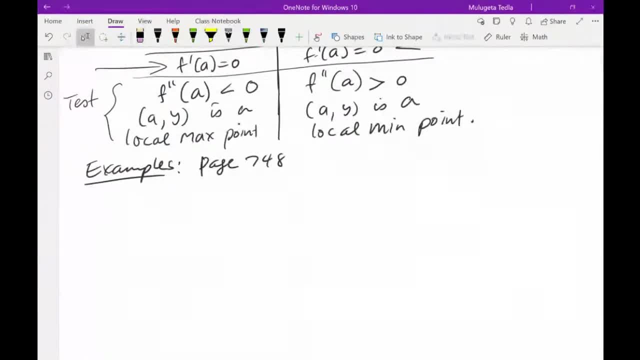 OK, So so number example: seven, eight, seven, four, eight, Number 15,, for example. So the question is: Why is given the same two X cubed Plus three, X squared Minus 36, X minus 10.. 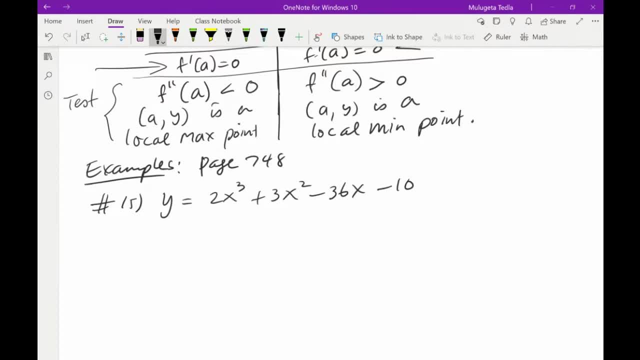 So they know, they want to know. you know we did the increasing and decreasing, We did critical numbers. Now they're asking: find the inflection points? Fine, I will. I'll ask you to find the critical numbers, Even though we did it. 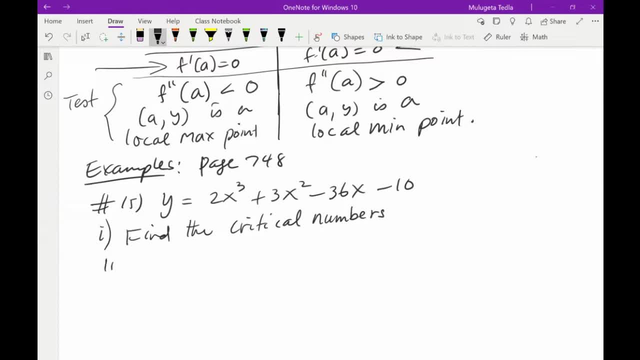 I'll ask you to find the critical numbers. Second, find the inflection numbers. Remember, I call inflection numbers, The book doesn't. I call inflection numbers The ones which are: X coordinates of inflection point, X coordinates of. 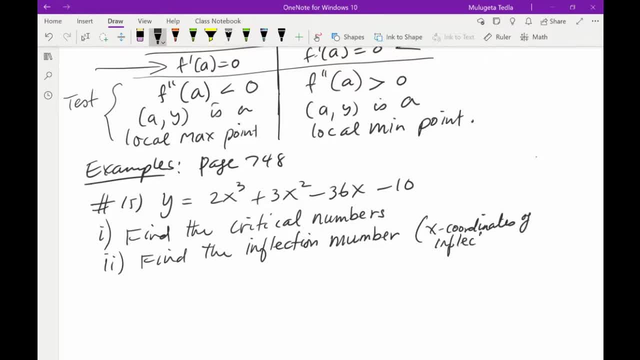 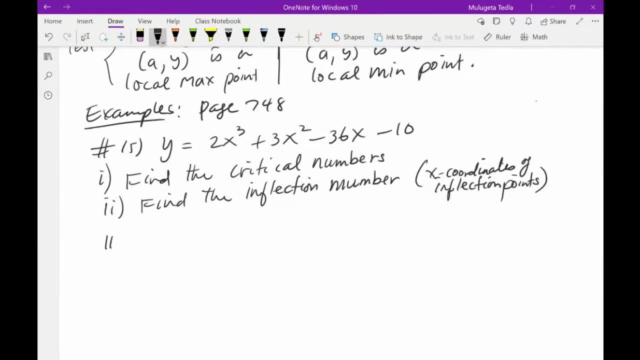 Of inflection points, OK. OK, The third case is OK If you find the critical numbers and then check Or test The critical numbers Using the secondary test before we use the first of using the secondary test For localization, For local marks. 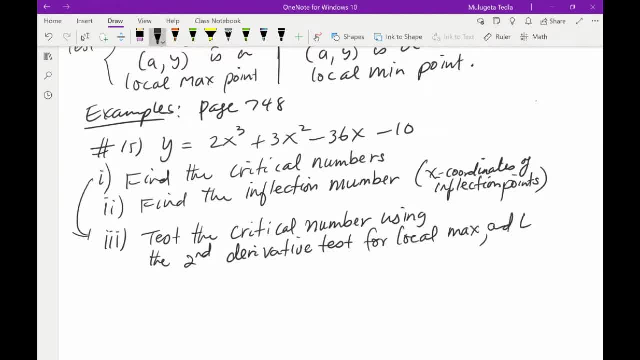 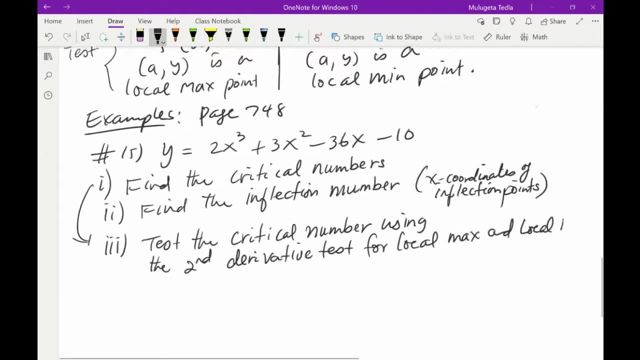 And local men. OK, We're going to do this. I can't write when it's close to the OK, So I hope you understand the question. So, solution: First of all, it's just like a summary, But we're using, for testing, a different test. 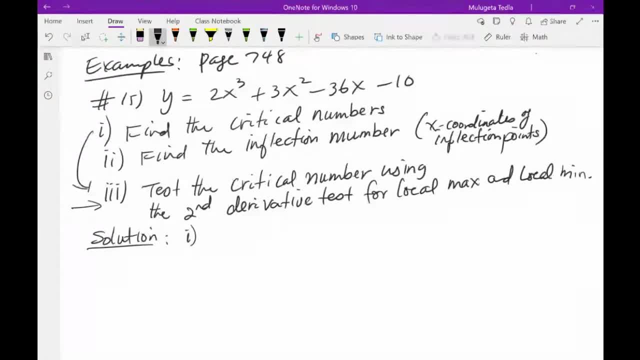 So we have the first Derivative equal to zero will give me critical numbers. This is a Principle, What we have found. When the slope equal to zero, Then we have a horizontal tangent, Horizontal tangent, Right. So what is the derivative? 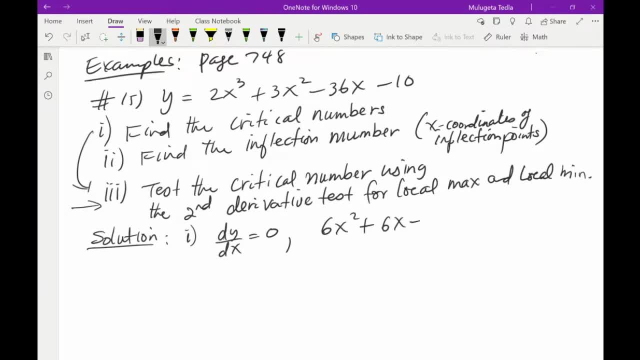 It is six X squared plus Six X minus 36.. Equal to zero. And we found, We factored this as X plus three and X minus two Equals zero. Then X equal to negative, three X equal to two, Where the 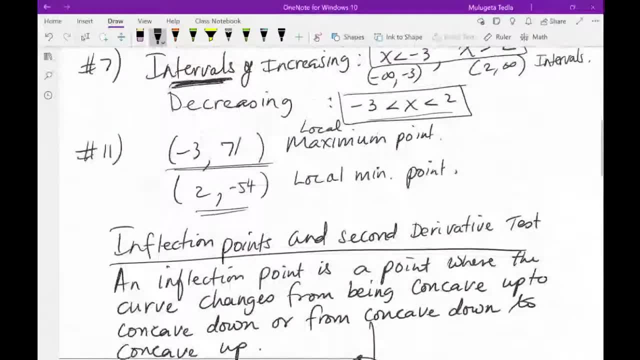 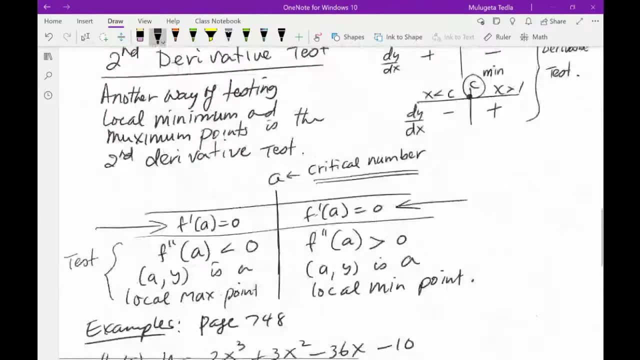 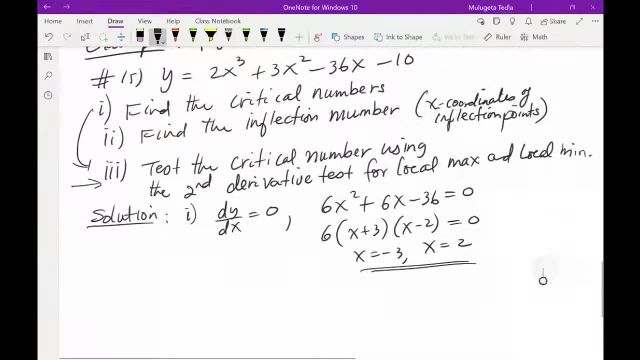 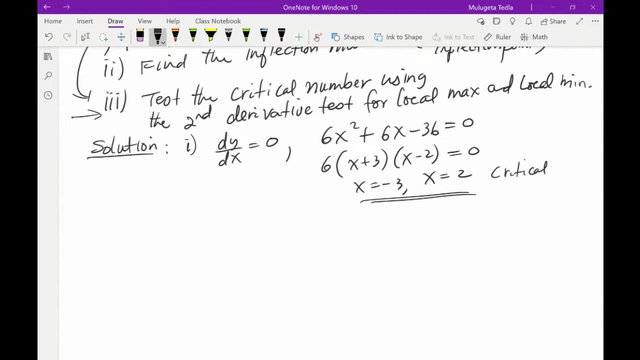 Critical numbers. Is that what we have in question? number seven: Yeah, Here Minus three and mine Positive two. OK, These are my critical numbers, Right? So I'm going to Also find. They ask me: These are critical numbers. 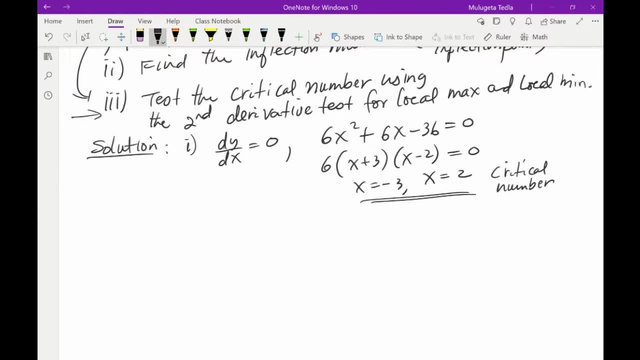 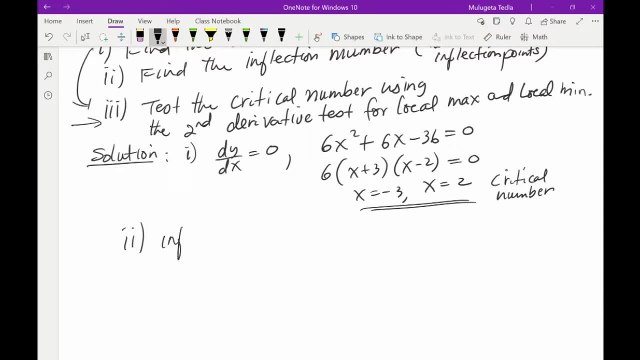 Now, Before I do test them, They are. Unfortunately I wrote it in such a way So I So I will go Find the Inflection point. The inflection point is: The inflection Number is Simply. 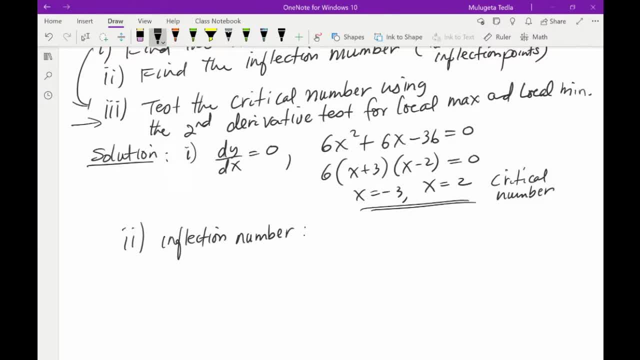 Just the same. Find the second derivative And let it to zero. It will give you a number. That number is inflection number. So, And What is the second derivative of this, Which is 12 X Plus six, Equal to zero? 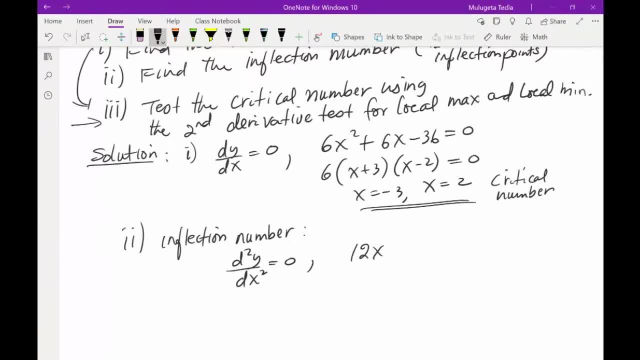 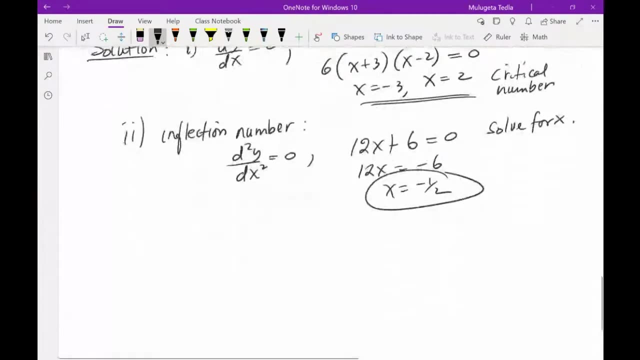 So That is The inflection Point. So X Equal to zero. So If you solve Solve for X, Then 12.. X Equal to negative six. X Equal to negative half, So X. 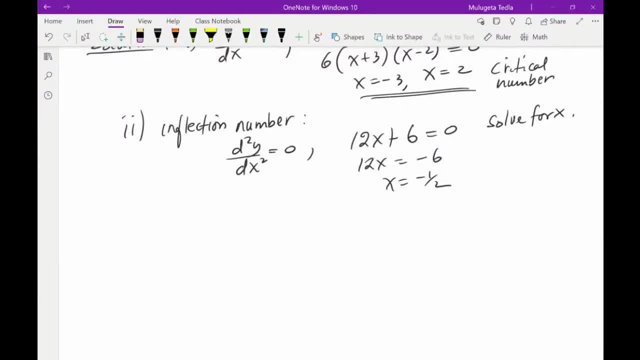 Equal to negative half Is Called Inflection number Or This Is Inflection number. Is An Inflection number Or The Inflection number Of The Graph? Here We Want. 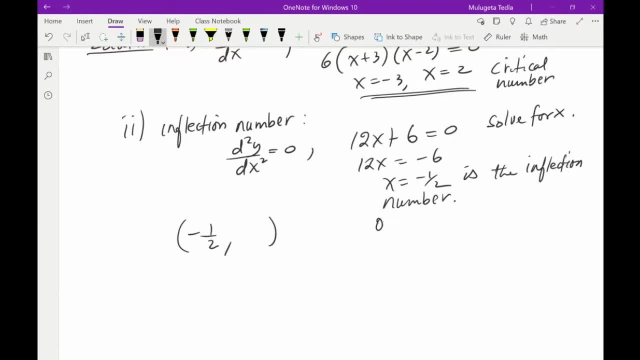 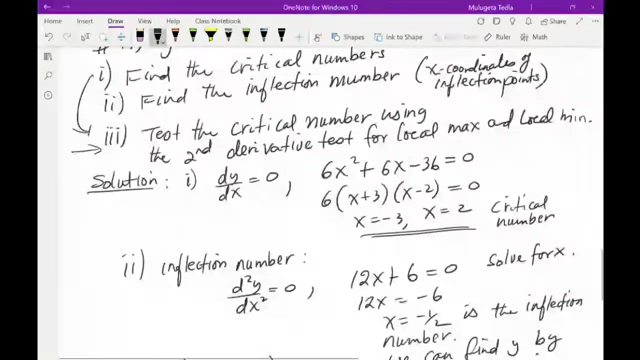 To Do Negative half. And What Is Y Y? Is You Remember Y? Or We Can Find Y By Plugging X Equal To Negative One Over. 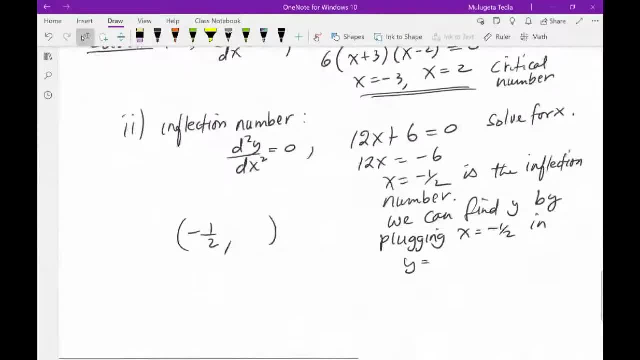 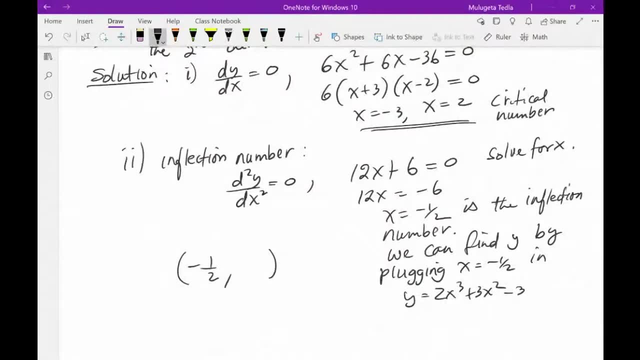 Two In Two X Cubed, Three X Squared. Two X Cubed Plus Three X Squared, Okay, Minus Thirty Six X Minus Ten, Okay. 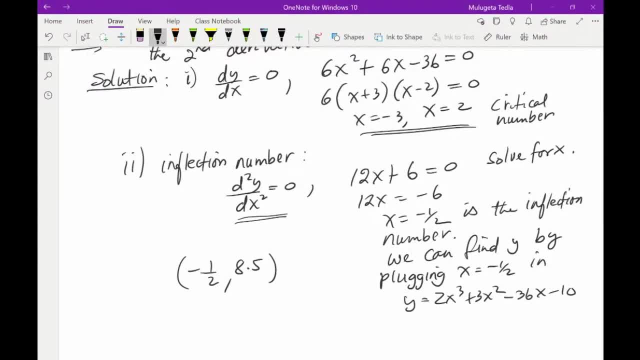 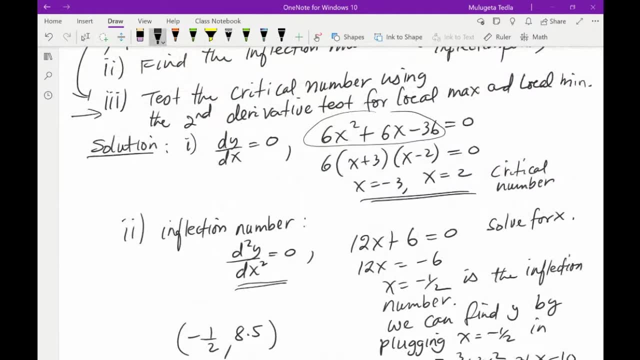 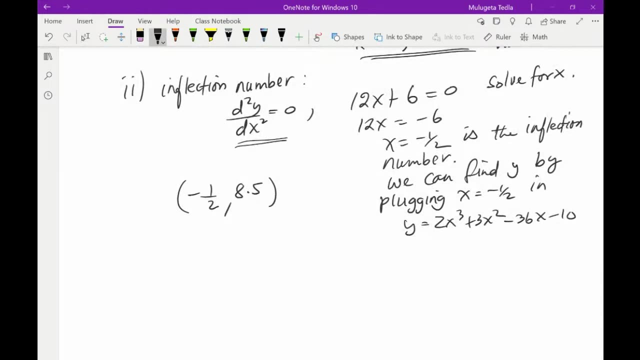 So Yes, Thank You So Much. Eight Point Of This Is Twelve X Plus Six, And Then When You Create It To Zero, You Solve For. 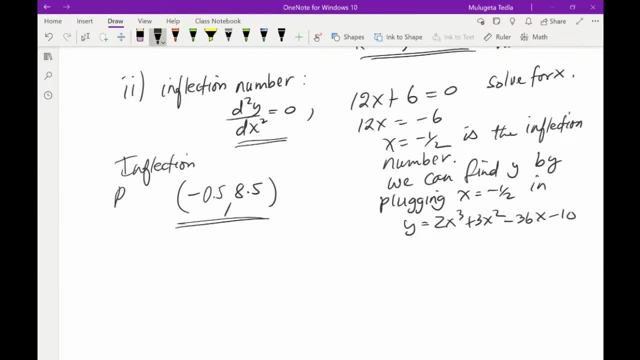 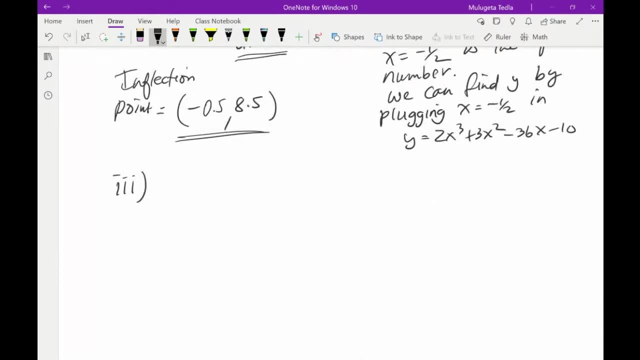 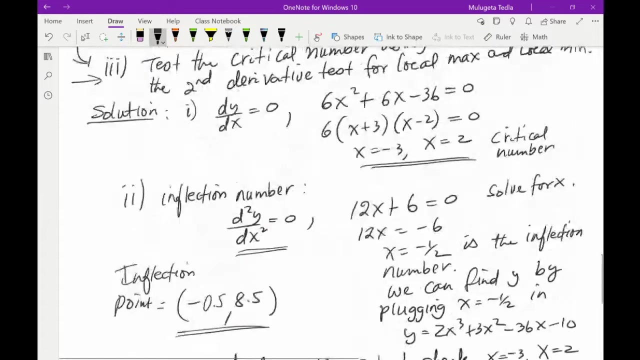 X, And Then You Get Point Five, Negative Point Five And Zero. Well, So So What We Are Doing Is Is To Check X Equal To 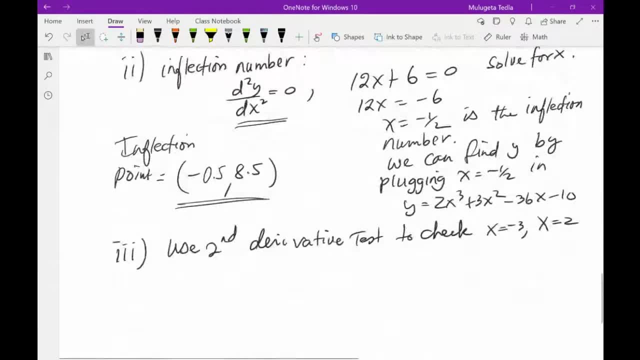 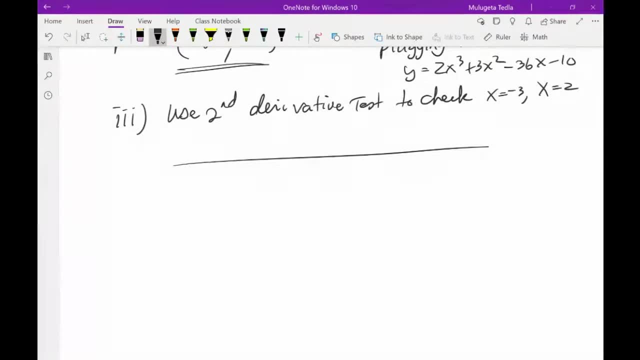 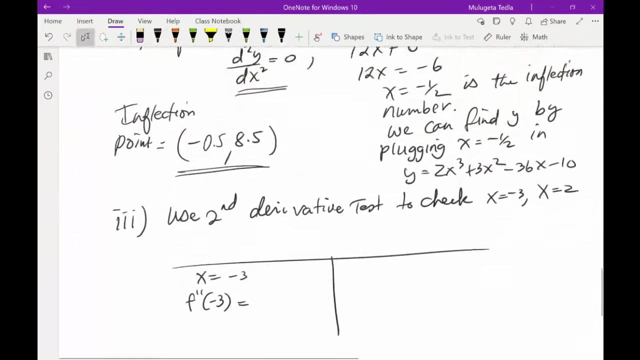 Negative Three And X Equal To Two, Because These Are The Two Critical Numbers, Say Negative Three. This Is My Test. What Is F Of F? 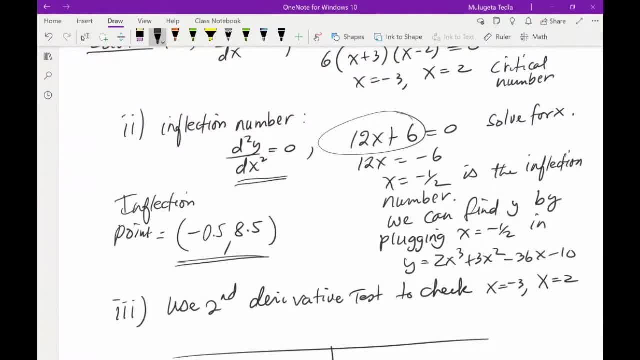 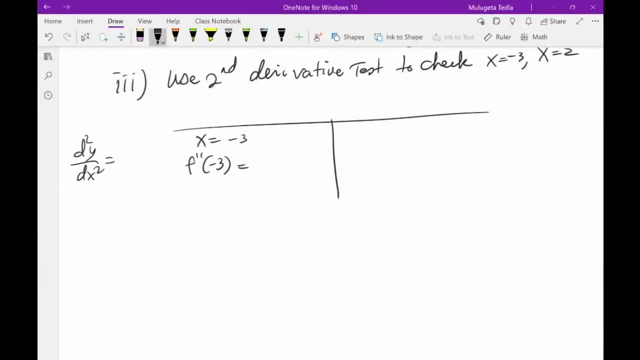 Double Prime Of Negative Three. What Is A Value Or The Sign When Negative Three Is Plugged Negative Three In, It Is Negative, Okay So 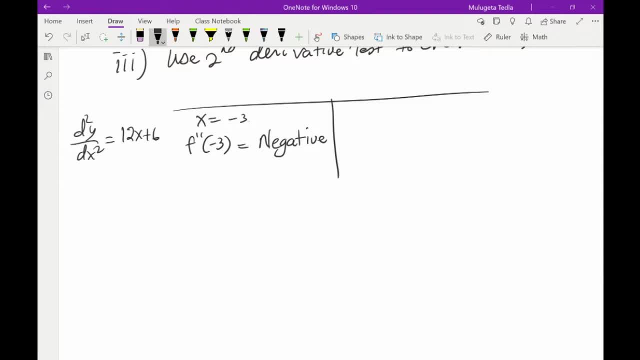 Twelve X Plus Six. When You Plug Negative Three In, There Is Negative Thirty. Six Plus Six Is Negative. Thirty Is Maximum Or Minimum. What Was? 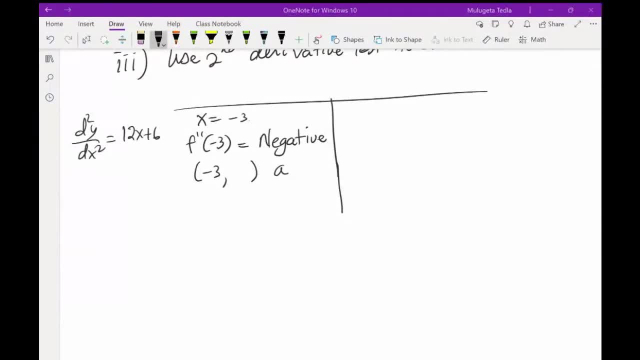 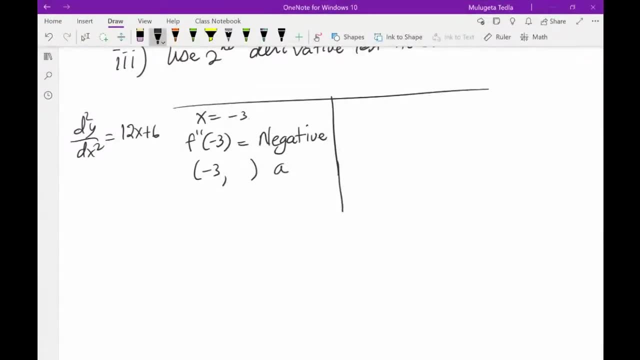 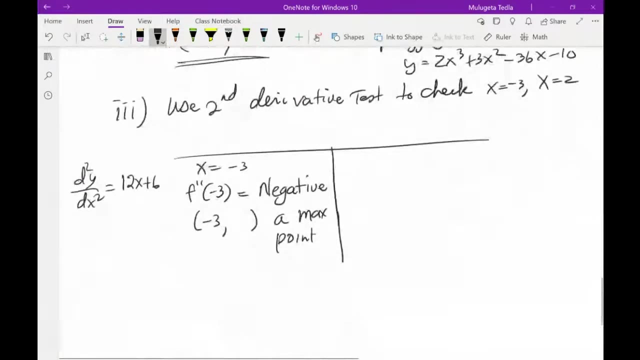 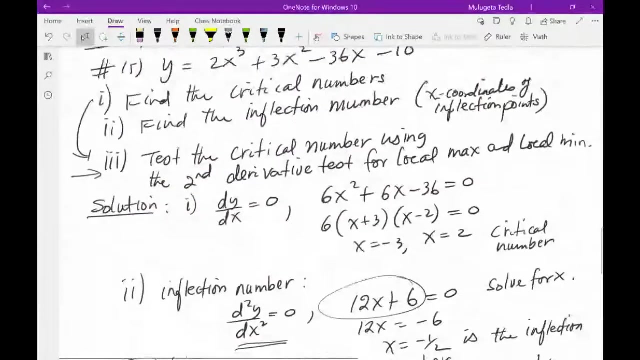 The Second Test Say It's Kind Of The Opposite. If You Get Negative, That Point Is A Maximum Point, Sorry. Maximum Yes, So Maximum Negative. 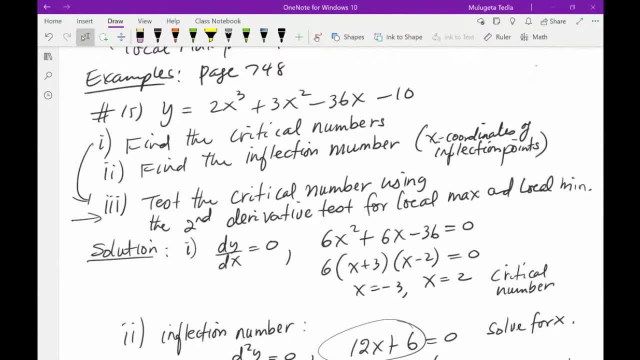 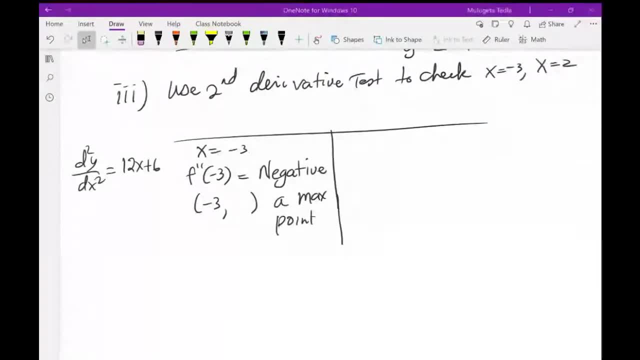 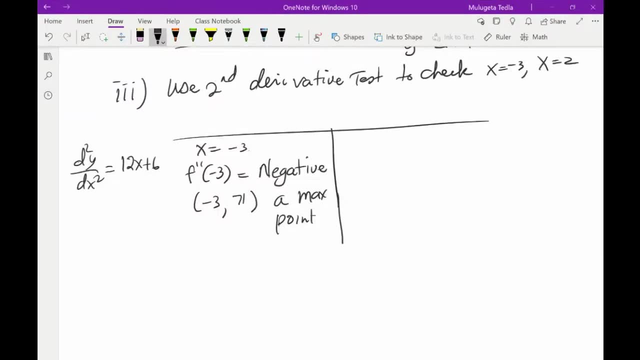 Three, So You Plug The Function Negative Three In. There You Found It. My Friend Is Being Helpful. Okay, It Is Seventy One, Very Good. 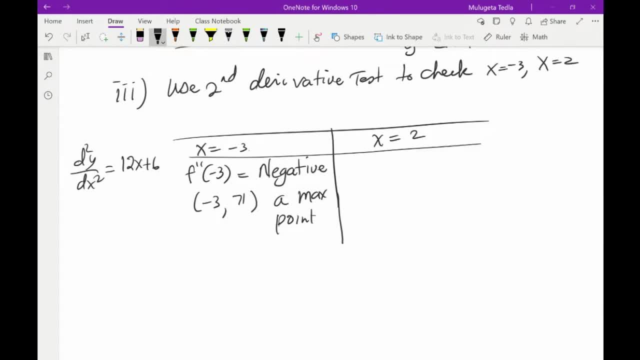 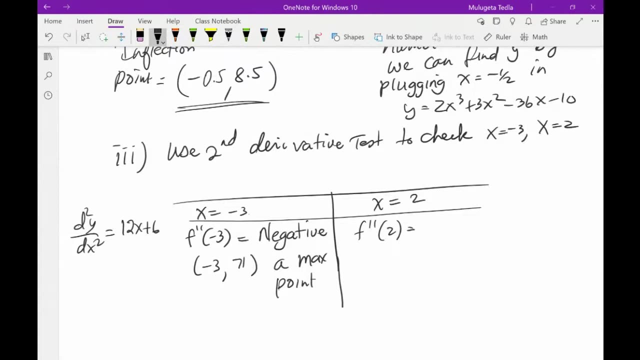 So Seventy One Minimum Point, But Let's Double Check. So F Of Double Prime Of Two Is What? F Double Prime Of Two Is This: 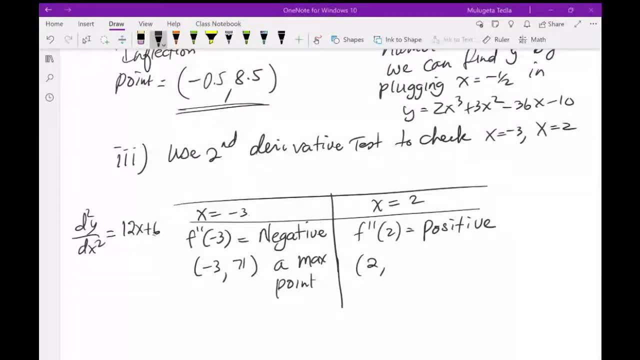 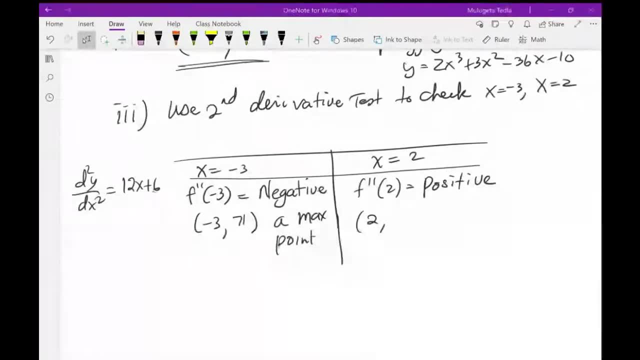 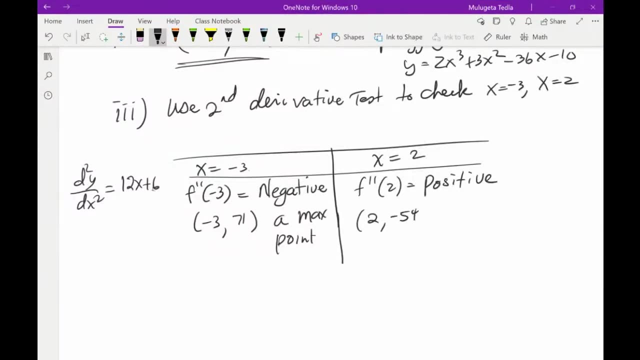 Is The Second Derivative Twelve Times Two Minimum Point. At Two We Found Negative Fifty Four. Right Yeah, Thank You So Much At Two And 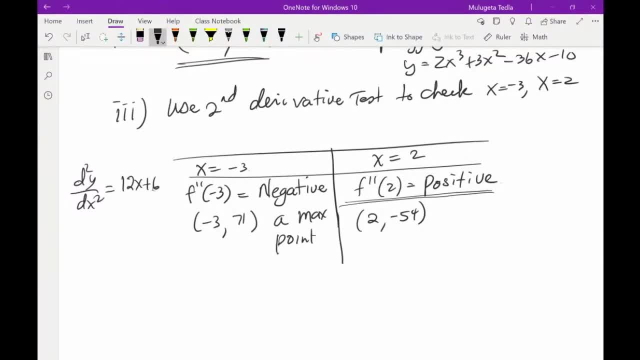 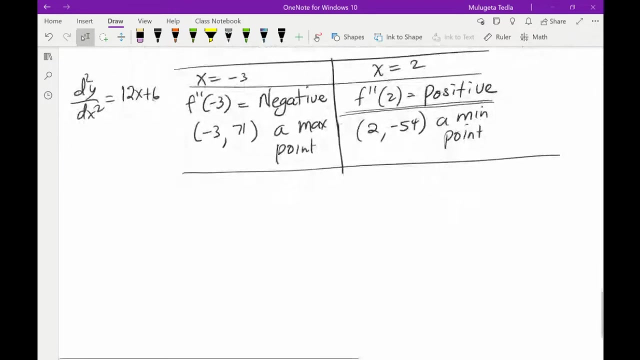 Negative Fifty Four. This Is What If The Second Critical Number Is A General, A General Rule Of Second Derivative Test. But What We Did? 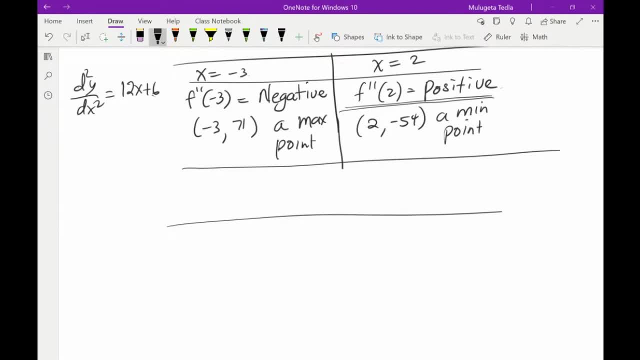 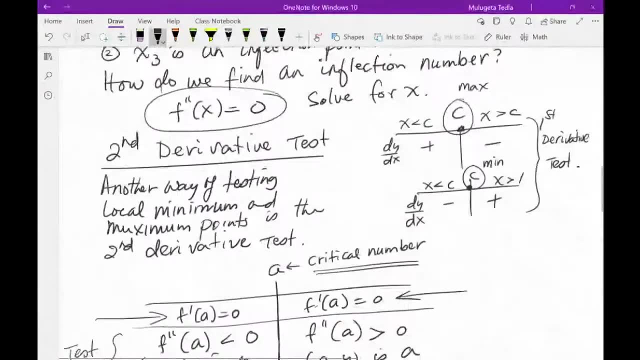 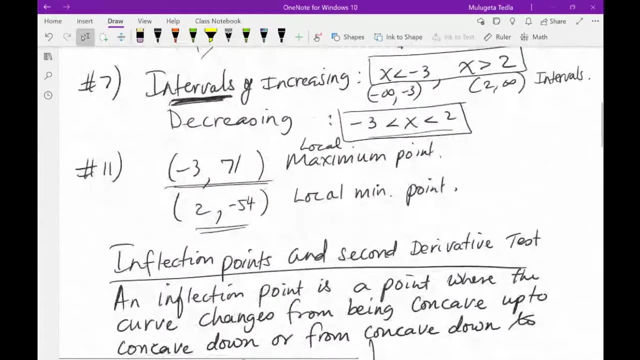 Last Time Was First Derivative Test Was Different. This Is The Second Derivative Test. I Don't Understand What We Have Done So Negative Three. 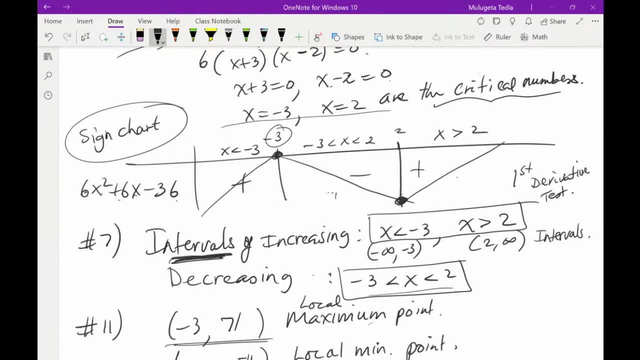 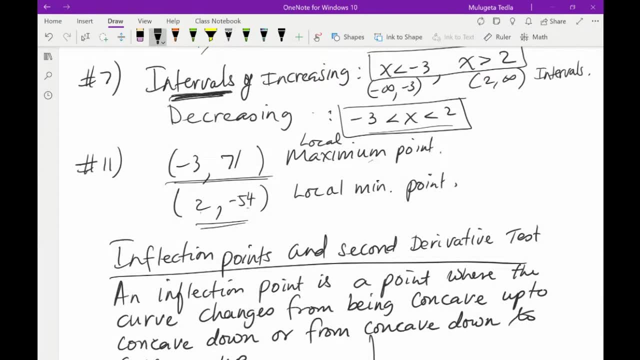 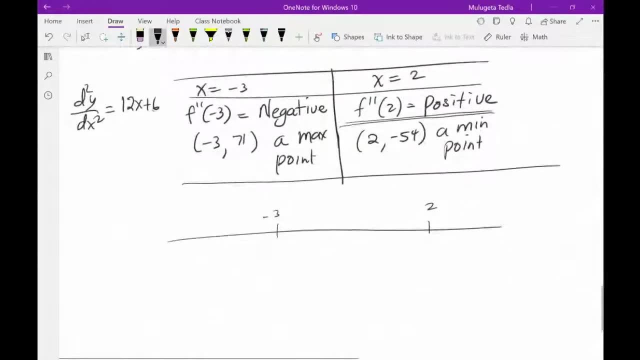 And Seventy One Is Maximum Point Two And Minus Fifty Four, And But We Used First Sign Chart, The First Derivative Is Minimum Point. 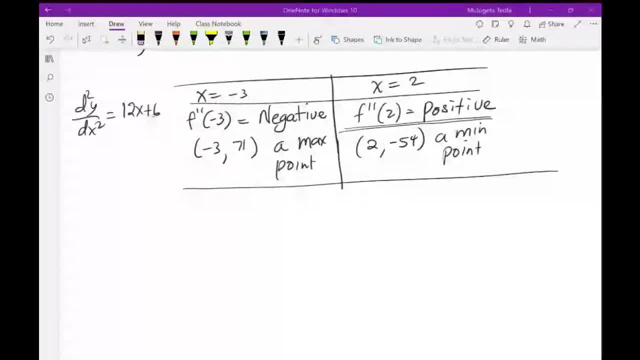 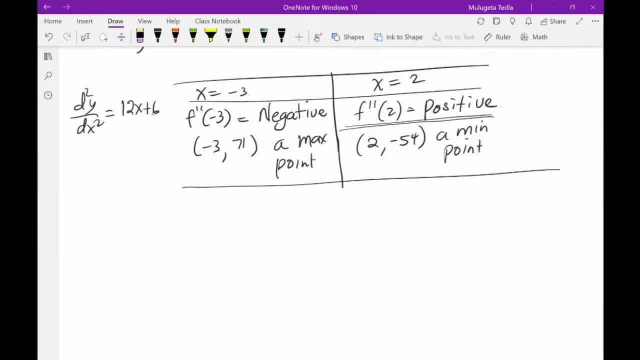 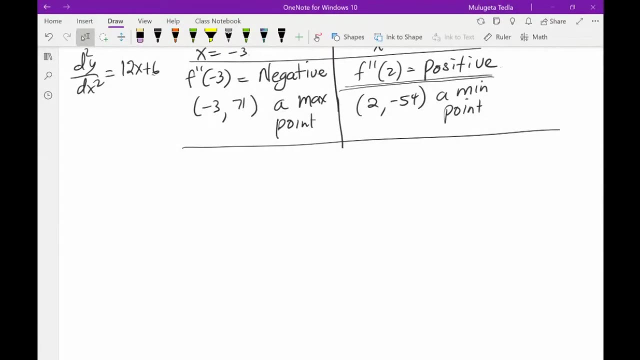 Okay, I Don't Have To Do It Again, But There Are Two Alternatives For You To Double Check Whether, Whether A Point, A Critical Number, 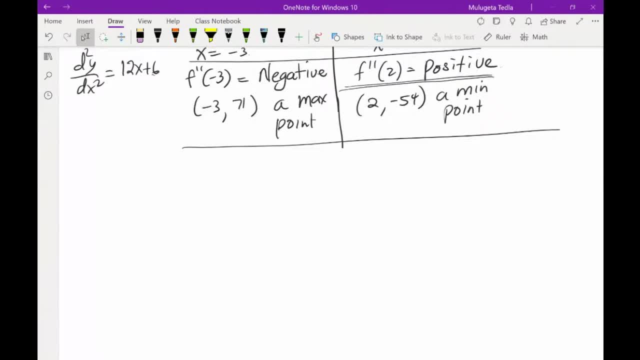 Is Local Maximum, Local Minimum, The Second Definition I Want To Use, The Second Derivative Is For Concave Up And Concave Down. Okay So. 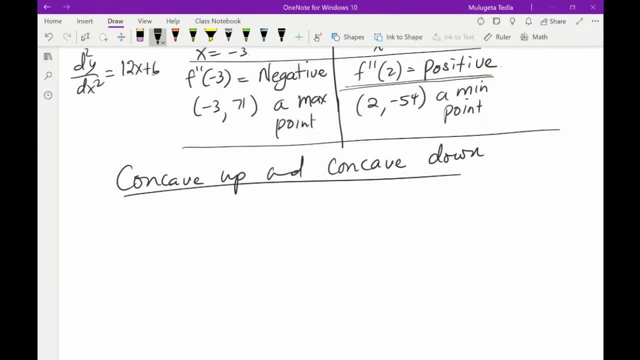 A Graph Is Concave Up When The Second Derivative. This Is How We Do It If The Second Derivative Of X, This Is Not. 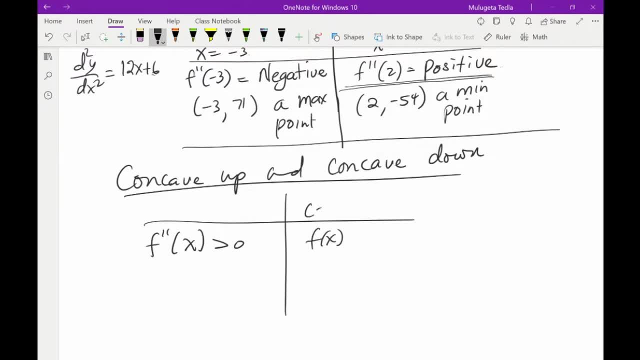 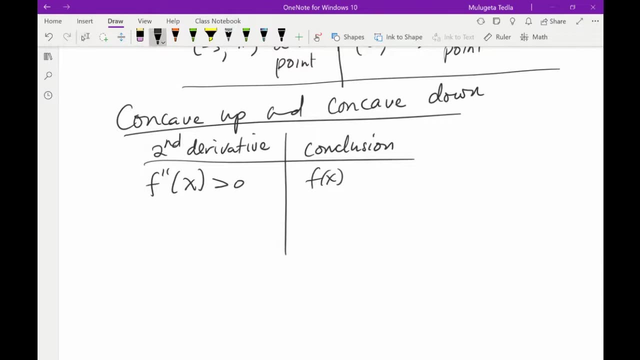 A Critical. Neither Critical Nor Inflection. If The Second Derivative Of X, Your Conclusion Is About The Function F Of X, So F, Double Prime. 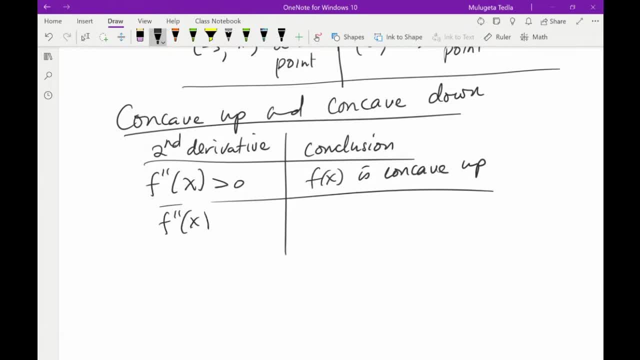 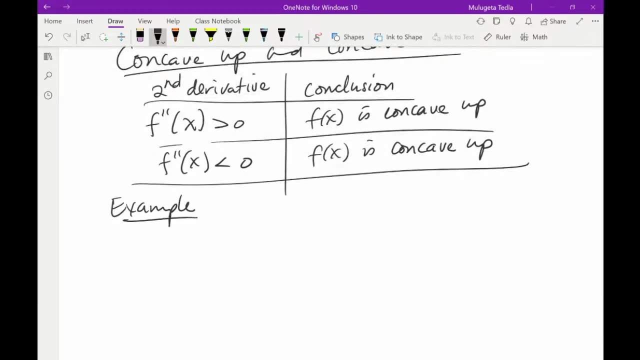 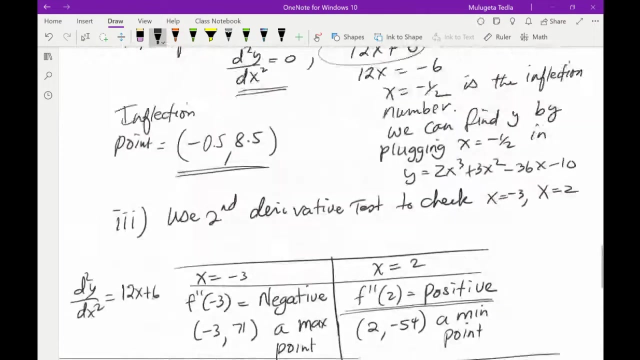 Of X Greater Than Zero, Then F Of X Is Concave Up. If, If The Second Example On On Number Fifteen Above, When Is A? 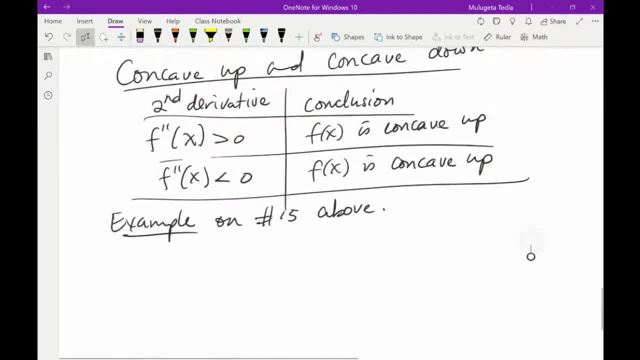 Graph Concave Up Or Concave Down Where? Okay, What Do We Tell? Can You Tell Me What We Could Do It To Find The Interval? 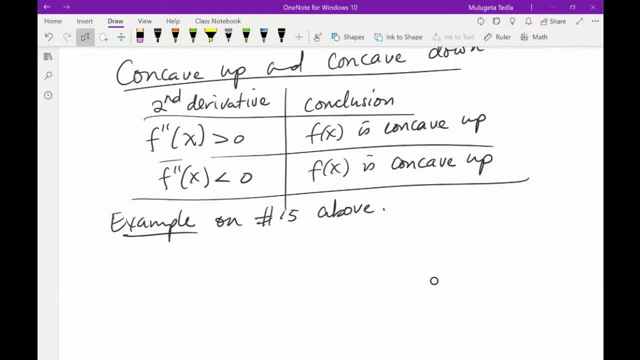 Of Concave Up Or Concave Down? We Don't. So It's Before And After. Yes, Exactly So. So What Would You Do? You Find The 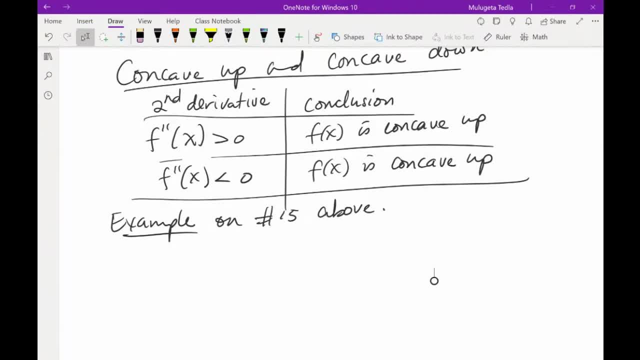 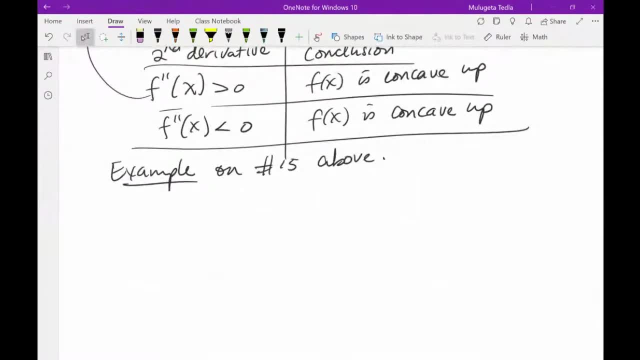 Inflation Point All The Time It Comes To Be. But What Is The Second Derivative? We Find The Second Derivative To Be This One: 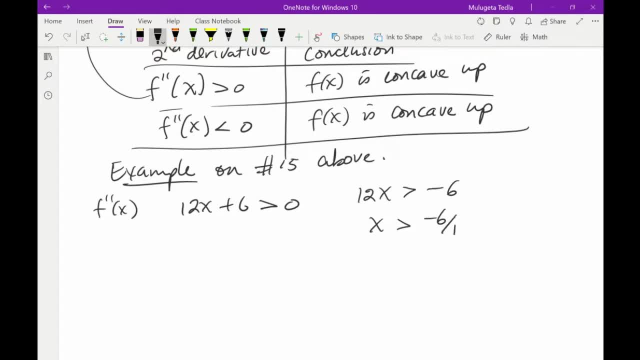 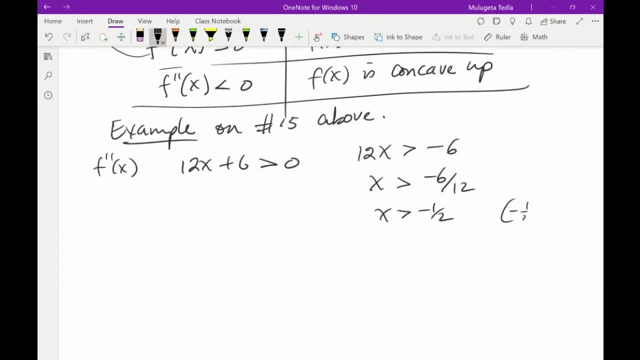 12x Plus 6.. So You Have The Interval Of Concave Up Is From Negative Half Up To Infinity, Or This. This Is Interval Of. 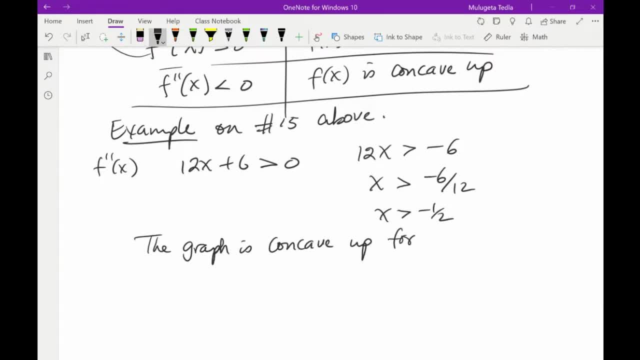 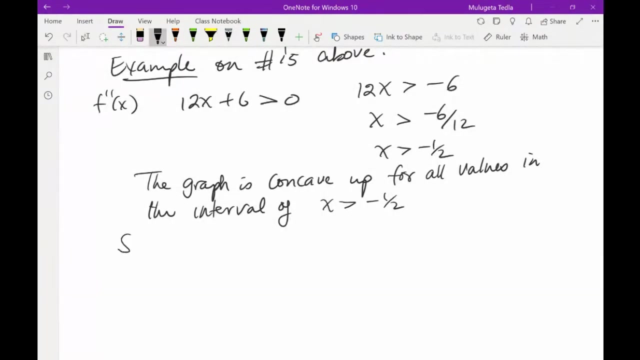 Concave Of The Graph. The Graph Is Concave Up For All. Okay, So If You Solve Also Similarly, If You Solve 12x Plus 6.. 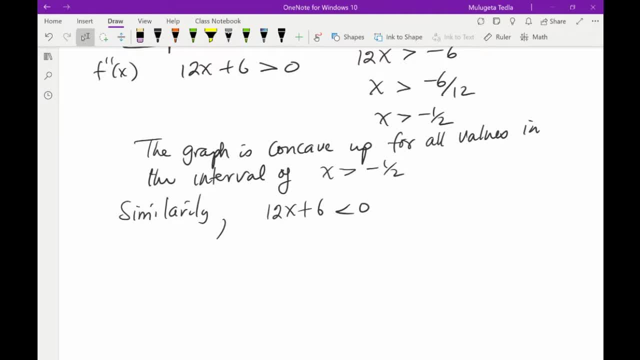 Less Than 0.. I Know Already The Chart, But If We Have Many Inflection Points, It's Good To Find It Like This: 12x. 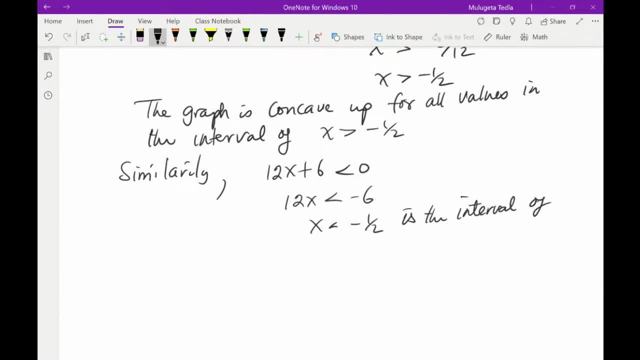 Less Than Negative 6. We Could Have Just Done It For The Inter Of The Graph, So We Can Sketch. Now Can We Sketch The? 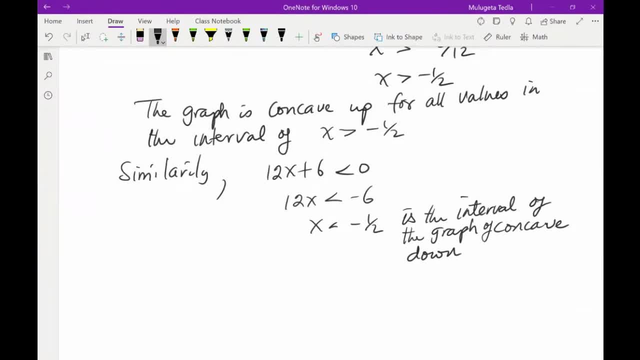 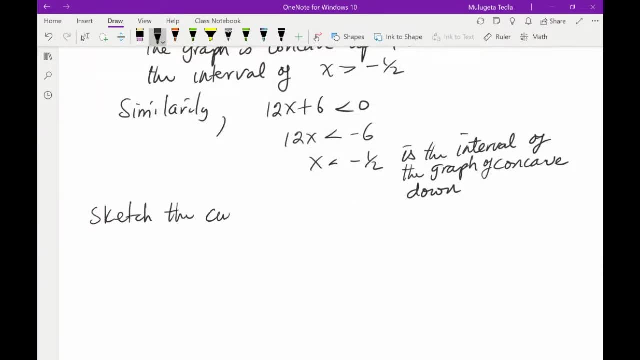 Curve. Sir, I Have One Also. One Question. Now We Say That If Double Prime Be Larger Than Zero, Right Yeah, And He, Here We Have. 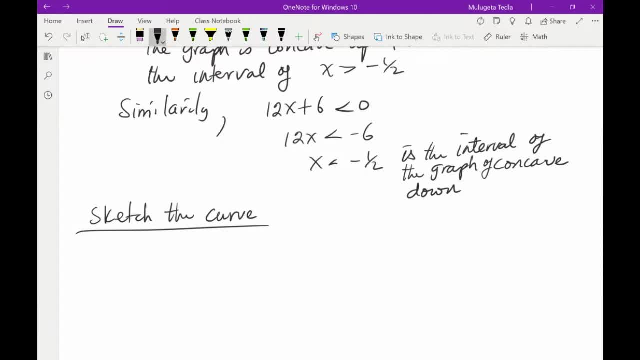 The Separation Is Minus Half. Still We Have Some Values. They Are Less Than Zero And The Concave No Kind Of. And Then Anything. 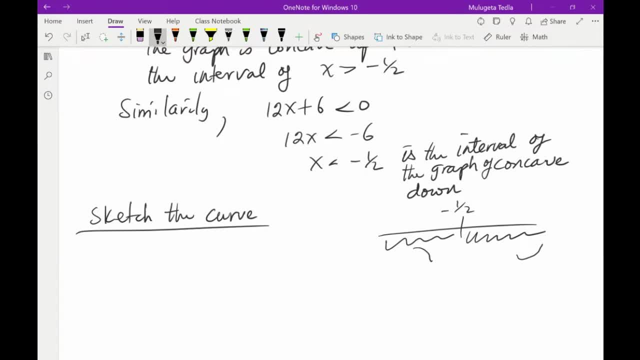 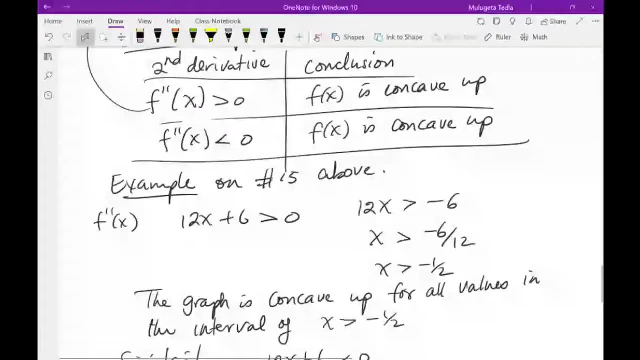 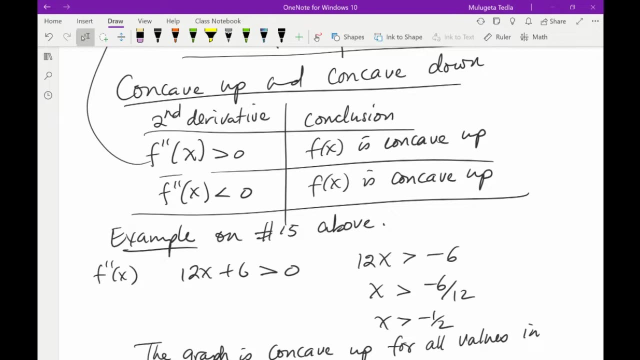 In Here Are Going Down Kind Of Okay. So If You Go To The Definition, Set On The Table That It's Up, Up If It. 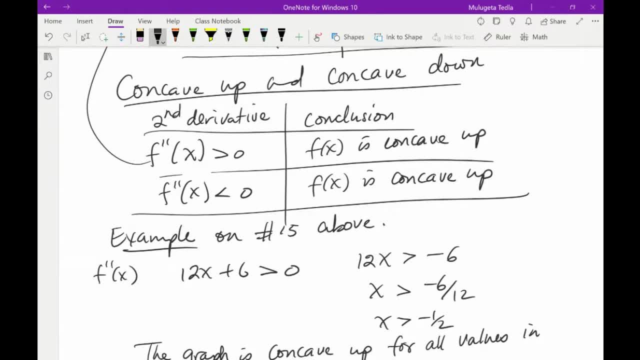 Is Larger Than Zero, But The System Will Produce An Interval, The Inequality. This Inequality Will Produce An Interval. Out Of That It's Not. 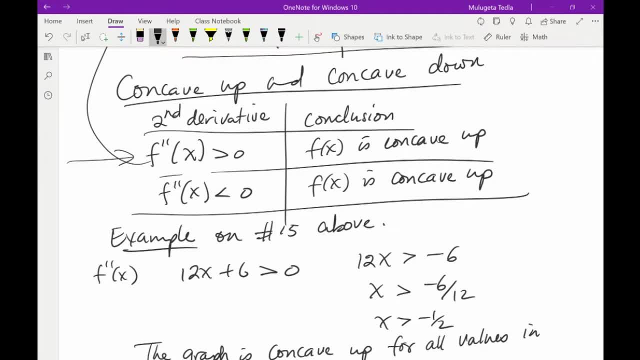 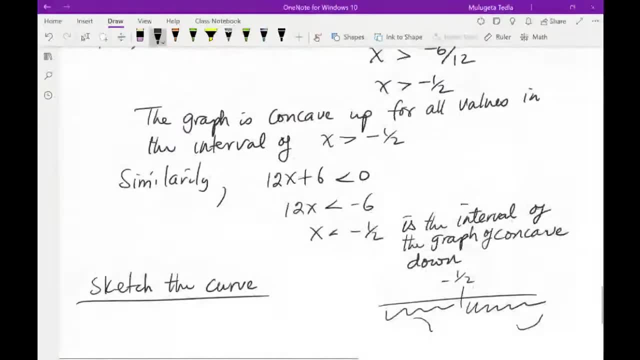 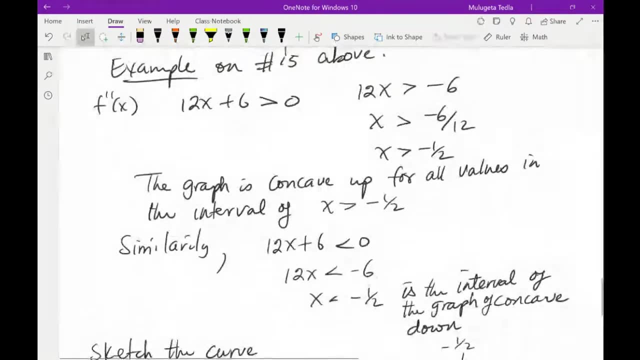 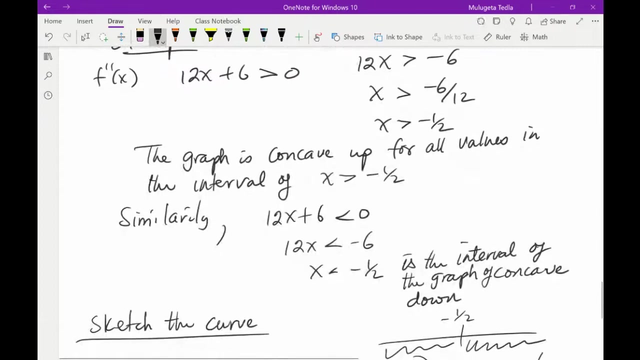 The Second Derivative Is High, When The Second Derivative Is Greater Than Zero And You Solve For X, This Is Okay. Okay, I Got Yeah. 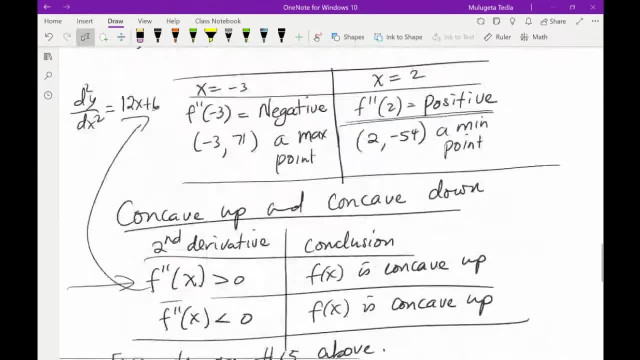 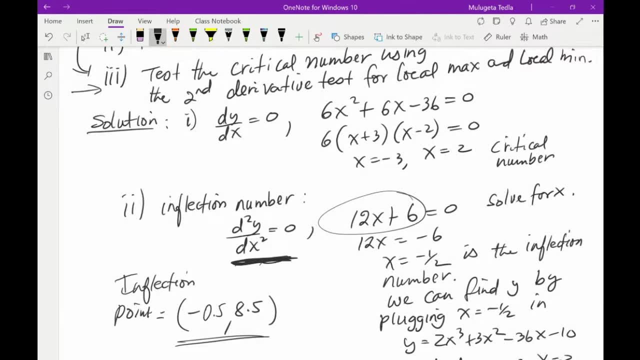 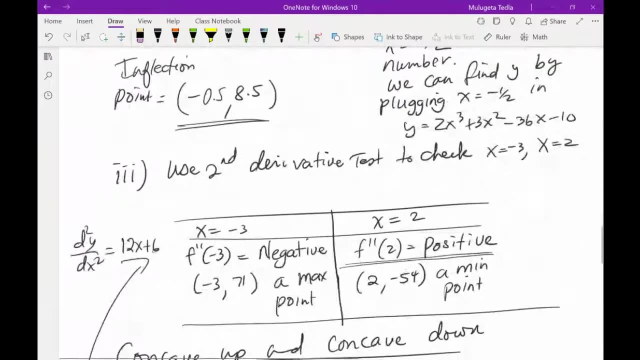 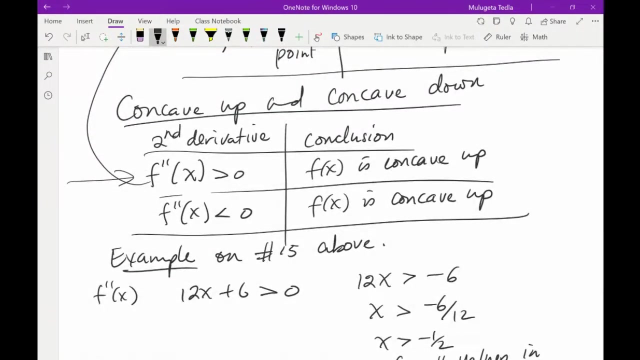 So The Inflection Point Has Nothing To Do. So That Is Comparing Numbers, Not The Definition. Okay, Yeah, Exactly. So When That? When We Have 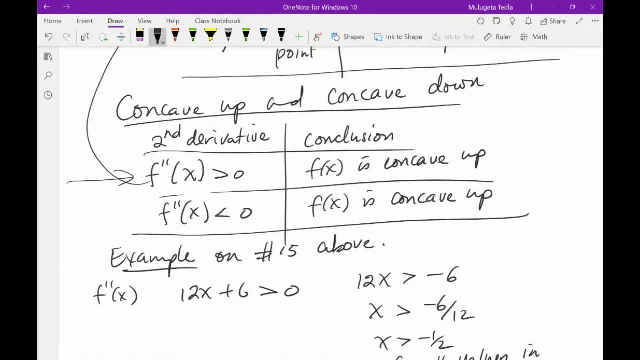 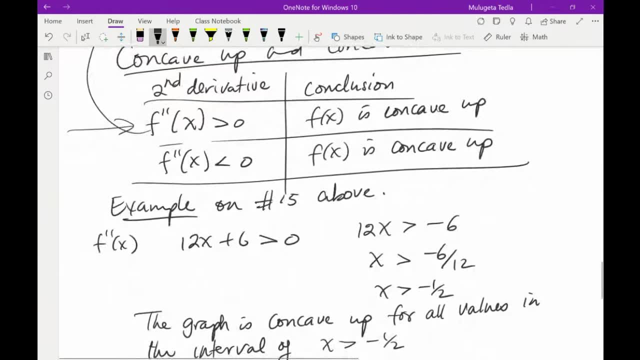 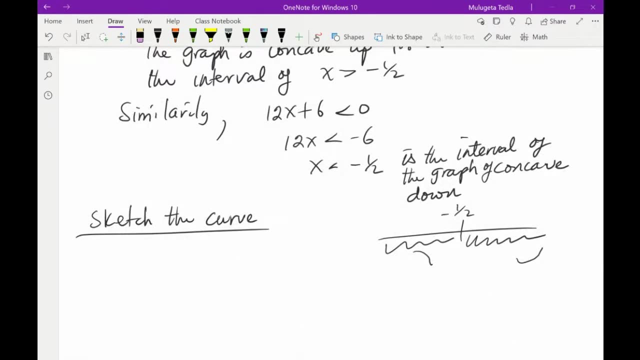 The Definition, It's Greater Than Or Less Than Zero. On The Definition, You Understand, Hopefully. Yes, Yeah, Yeah, Okay, Very Good, But But The Result? 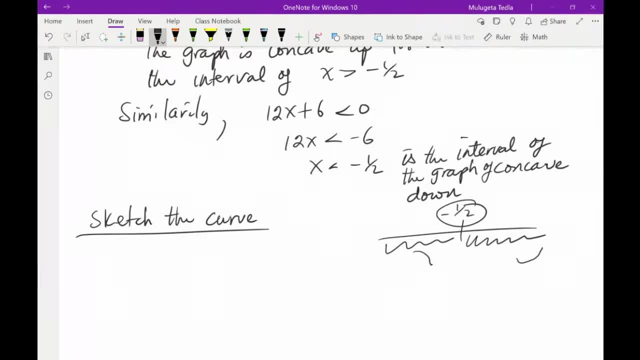 Will Bring You To Negative Half Still, You Know, Because It's At The Negative Half Which You Understand. But A Inflection Point Is A Boundary. 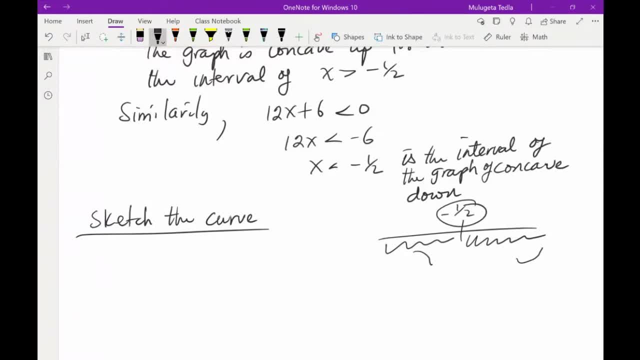 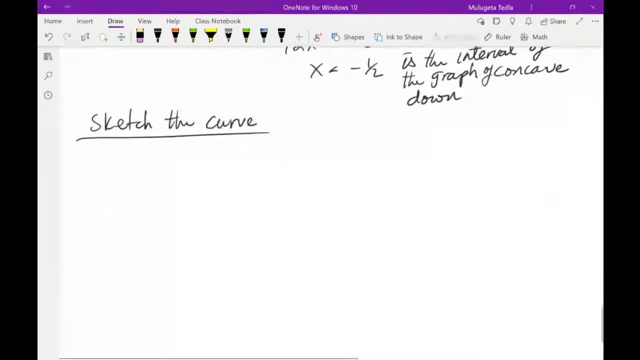 Of Concave Up, Concave Down. Okay, So I Know You Could Do It Again, And So So What Is A Result Of Negative Three? So 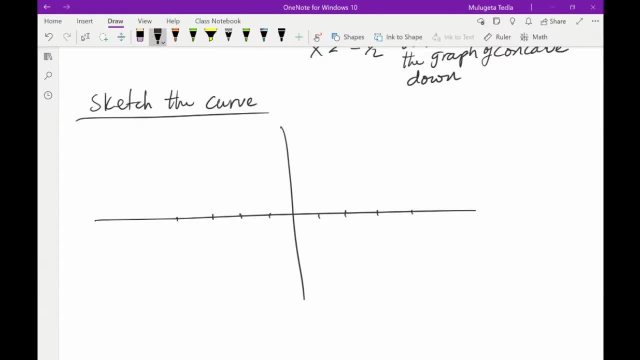 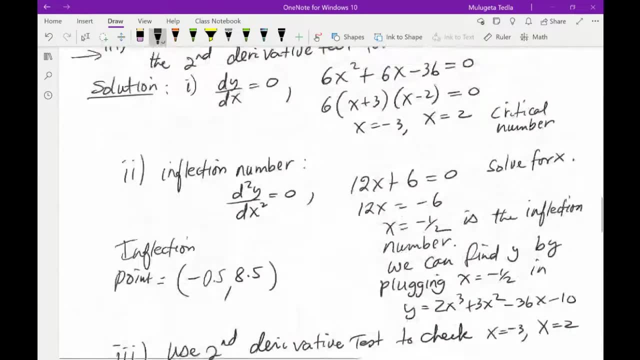 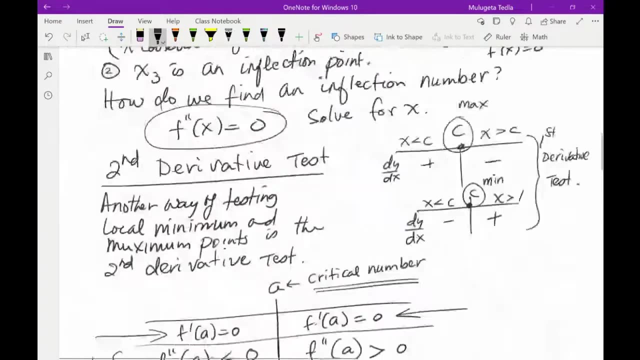 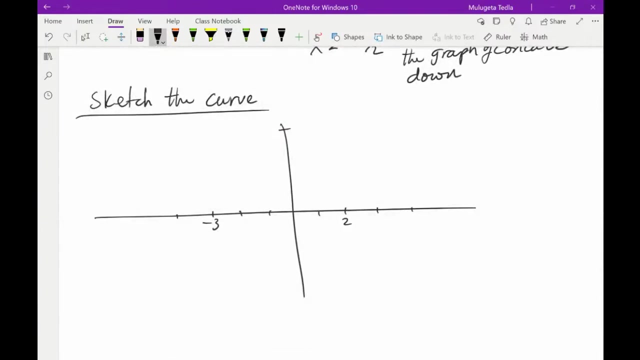 One, Two, Three, Four. Negative One, Negative Two, Negative Three, Negative Four. So I Have Two Here, I Have Negative Three. What Is The Seventy? 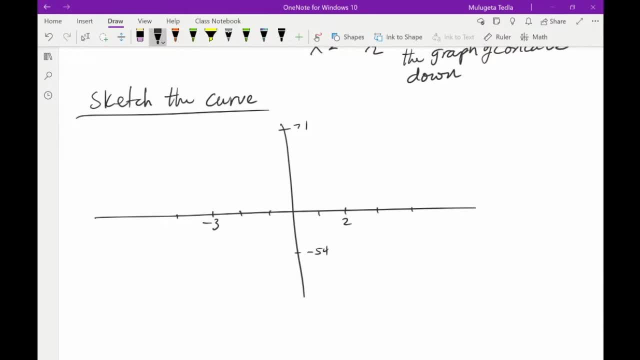 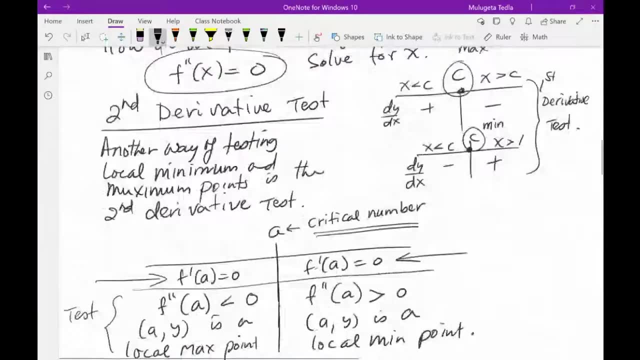 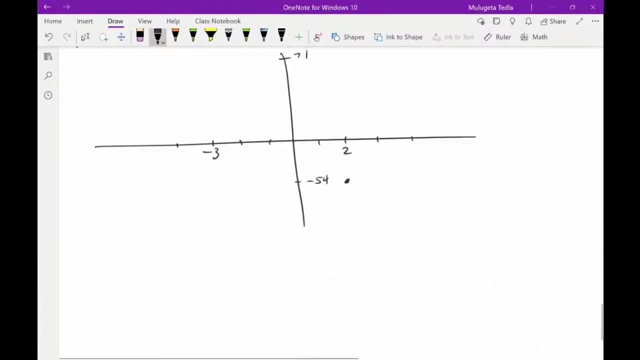 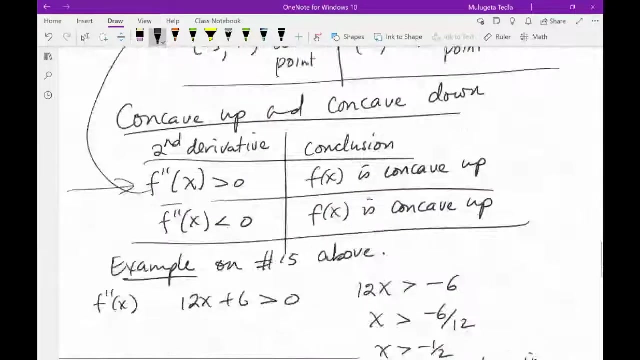 One Here Is Negative Fifty Four. So At Two, What Do We Have Class? At Two, We Get What Minus Fifty Four, Minus Fifty Four. 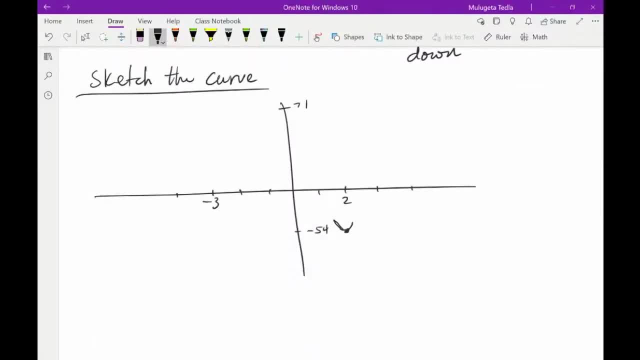 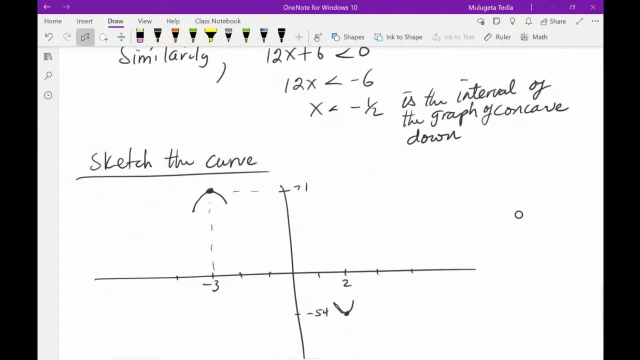 Thank You. So I Have Negative Three And It Is Seventy One. It's Maximum On Negative Three, And Seventy One It's Maximum On Negative. 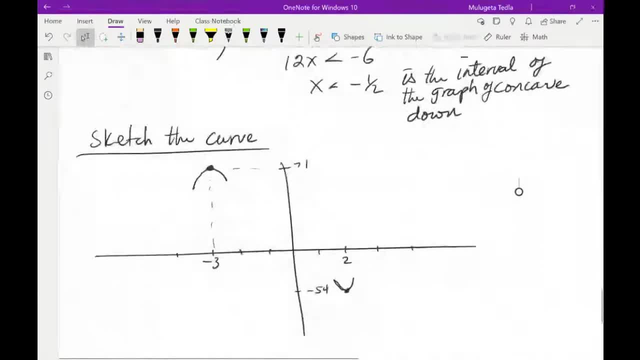 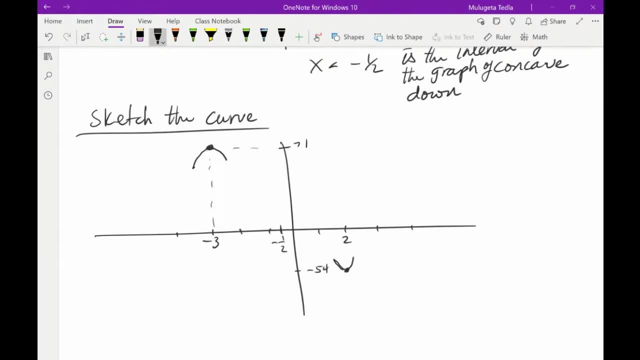 Three And Seventy One. It Is Maximum, Here Negative One Over Two And Eight Point Five. Yes, Eight Point Five, Some Somewhere Here, So So, 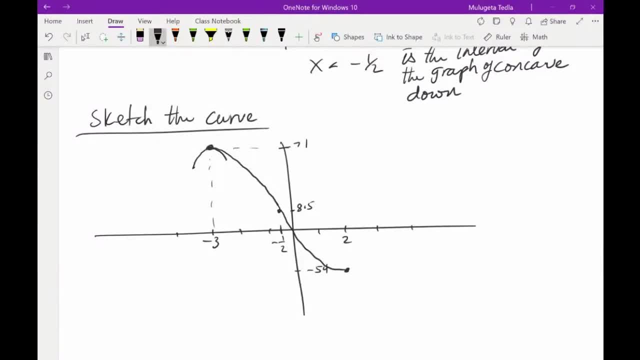 It Is Going Down Up To This Level, But It Just Shows, Yeah, I Had It The Better Way The First Time. Okay, So This Is. 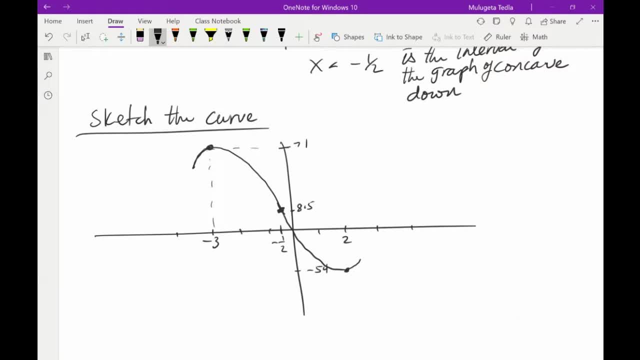 Going Up, Going Down, Because It's Maximum, Minimum And Inflection Point. I Think We Should Find X Intercepts. It Should Be Newton Method, It's. 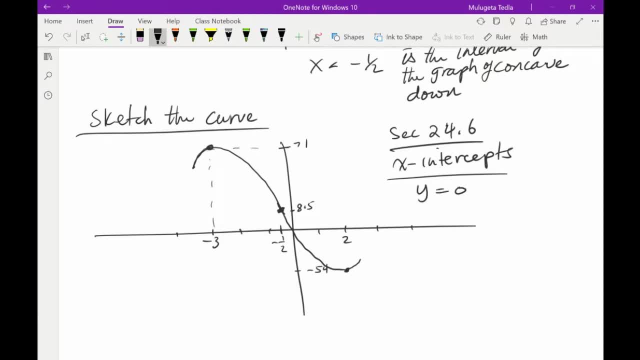 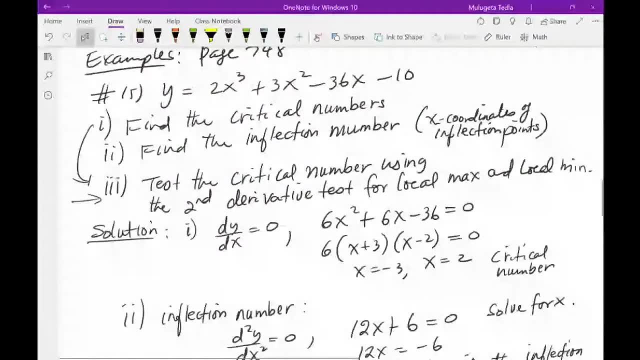 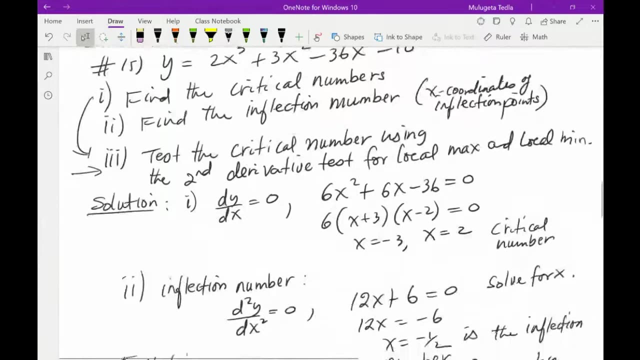 Very Okay, Newton's Method, But We Can Use It Straightforward. Y Equals Zero, Right, These Are. This Is, I Think, One They Wouldn't Give. 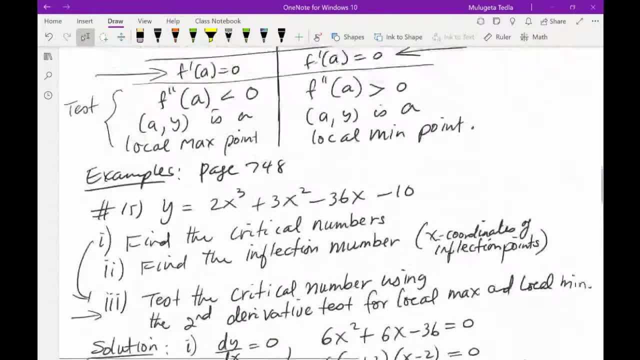 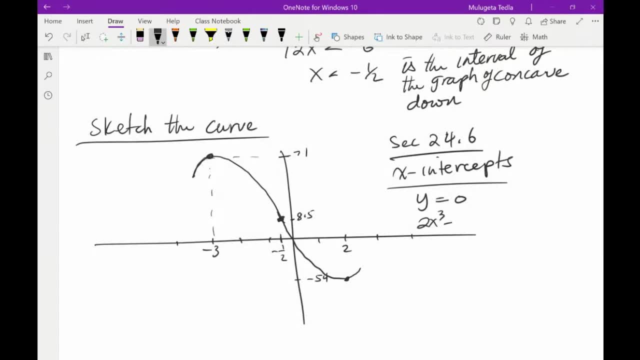 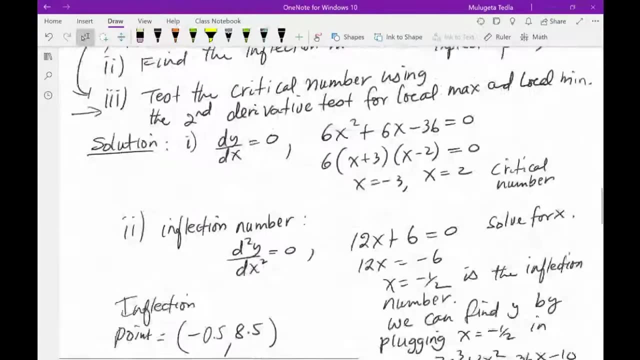 Us A Difficult One. So So, Technically, I Have To Stop Here Because I Don't Have Time. But Really, Two X Cubed, Three X. 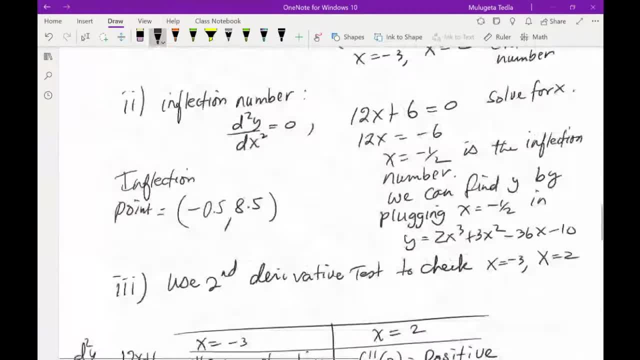 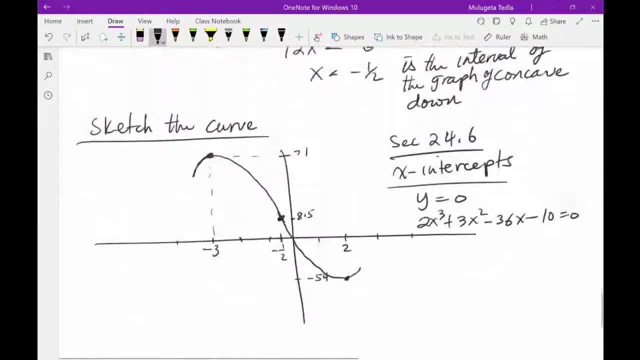 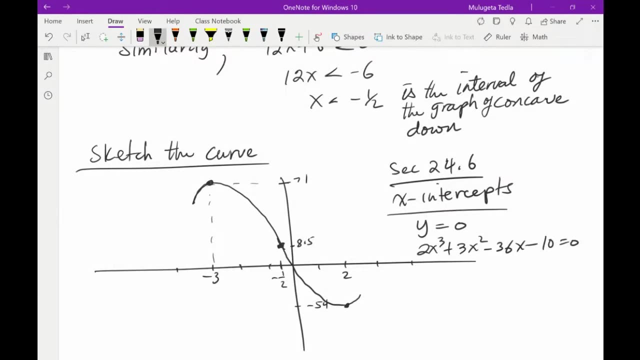 Squared, Two X Squared. So Yeah, Minus Thirty Six, Minus Ten. Okay, So Is It Really Like Two At Three? Yeah, Probably, You're. 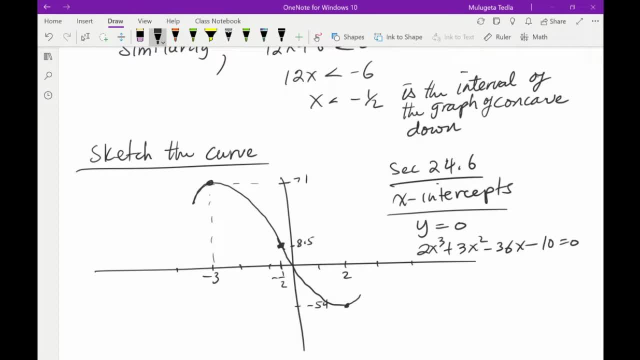 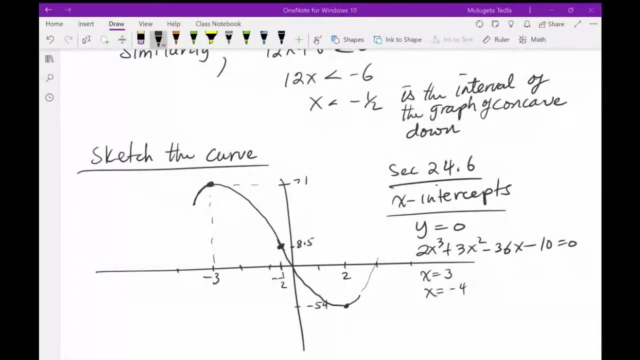 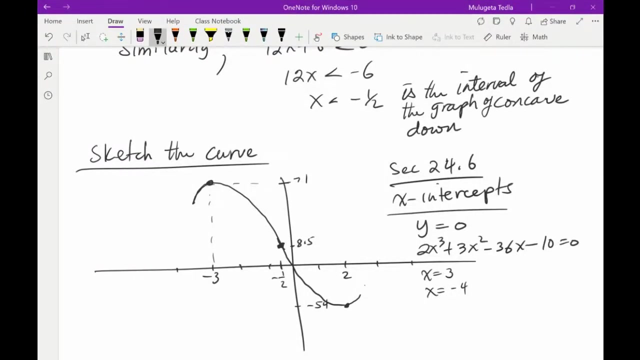 Right, So We Probably Have. If We Don't Know, What Is It Zero? That's How We Chat, Because Is It Going? Yeah, Yeah, Okay, Thank you.